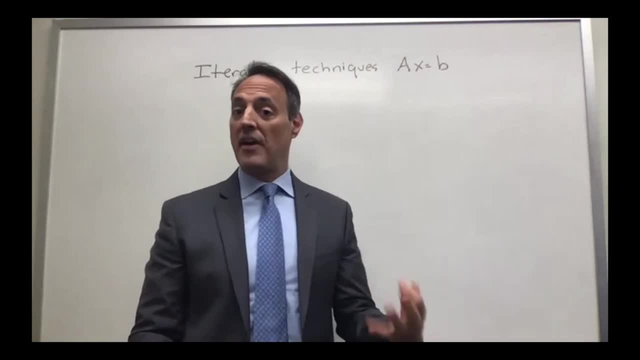 revolves around AX equal to B, And so what we're going to do is we're going to do a little bit of thinking, So iterative techniques for AX equal to B, And so what we're going to do is we're going to decompositions of A, which, again, the decomposition lets us solve AX equal to B. 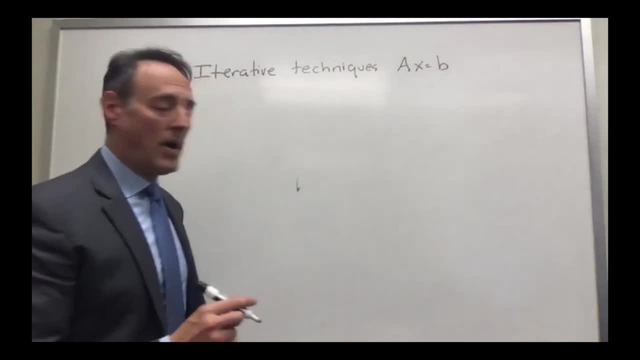 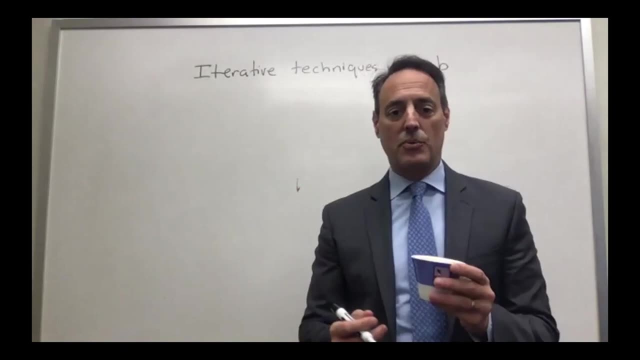 okay, or lets us characterize A. So I'm going to start off with a simple example And I'm going to just show you. we're going to start off by writing some code actually. So we're going to do a little bit of MATLAB today and just do some little bit of iterations to try. 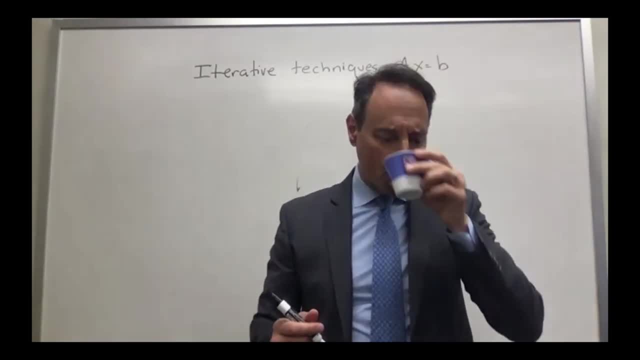 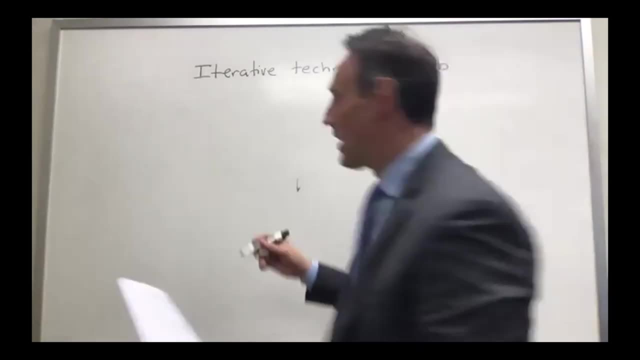 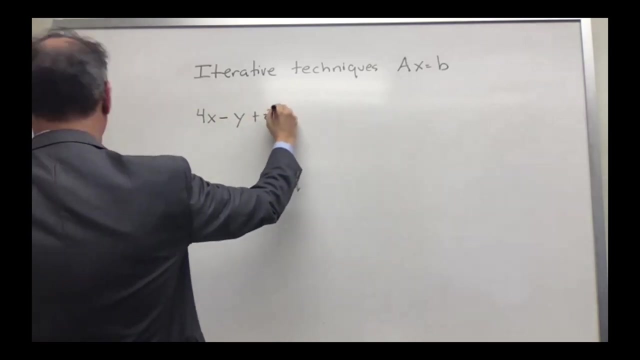 to solve some very basic AX equal to B problems. So I'm going to start off here with a simple problem, Which I'm going to write as follows. It's a three by three system: 4X minus Y plus Z equals 7.. 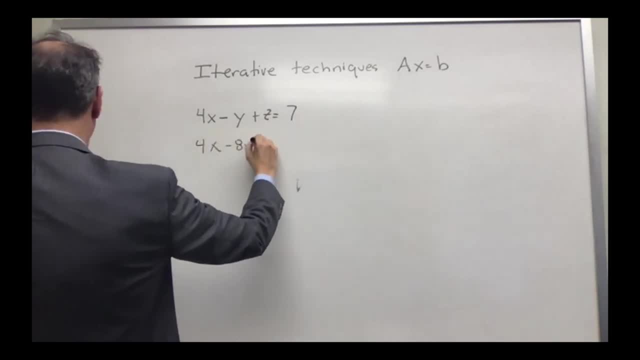 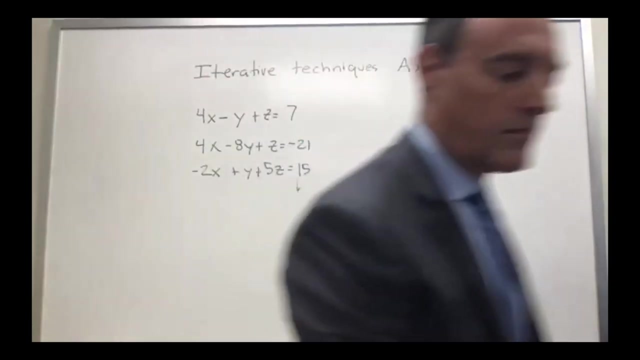 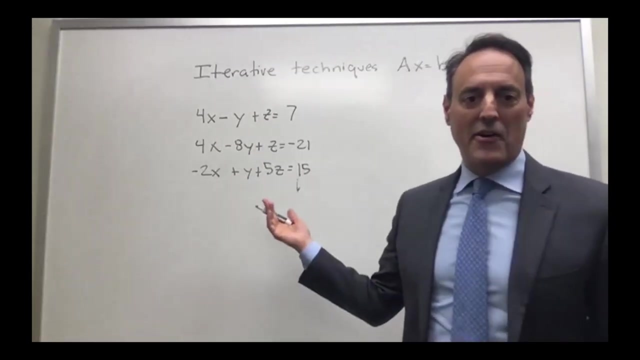 4X minus 8Y plus Z is equal to minus 21. minus 2X plus Y plus 5Z is equal to 15.. Okay, so that's our system: Three by three, system of equation, And this is not that hard. 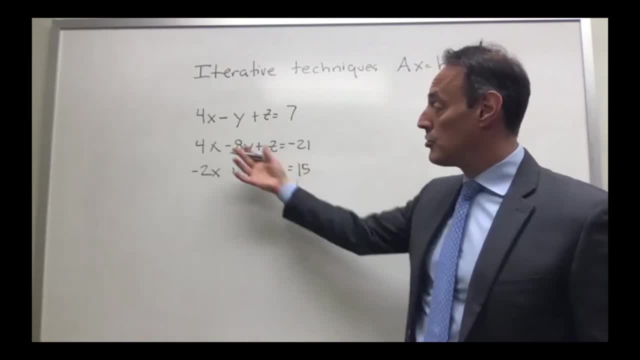 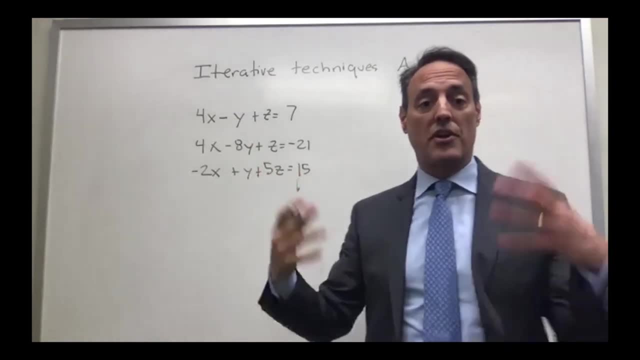 to solve right. So in some sense, if you're going to solve it, you could do Gaussian elimination, LU decomposition, whatever you want to do. You could do this one by hand. You put it in as sort of the you know you, whatever. Gaussian elimination is a very simple way to do this one. 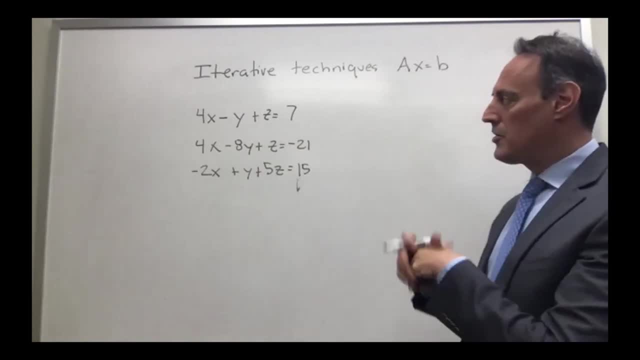 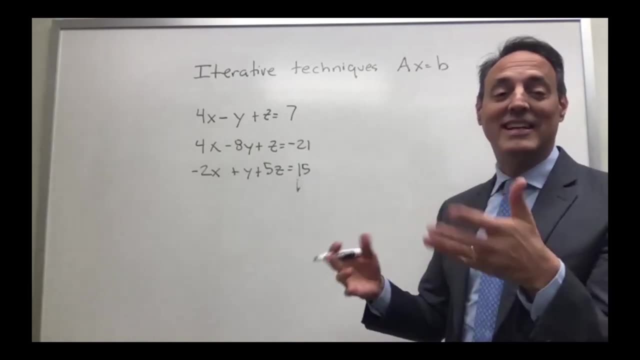 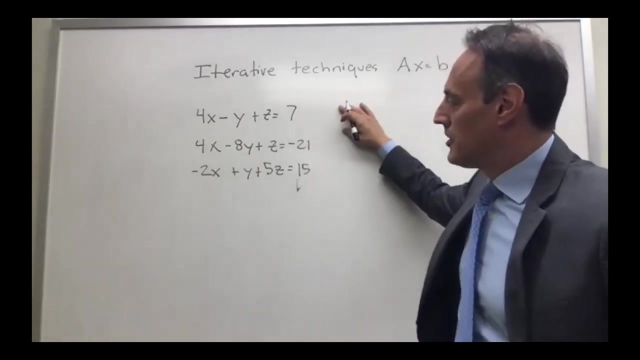 But I'm going to change the way we do this. now What I'm going to do is something interesting. Well, I mean, interesting is a relative term, but let's just play along as if this is really interesting. what I do next? What I'm going to do is say: okay, from the first equation I'm going 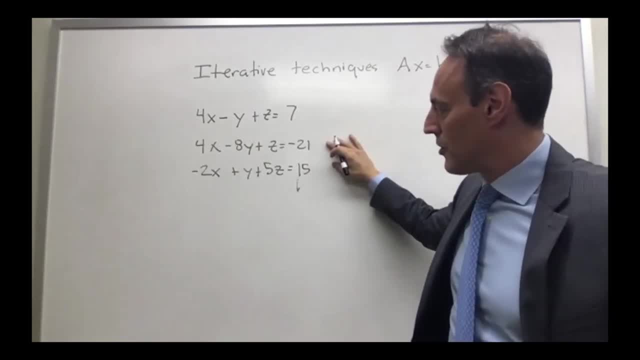 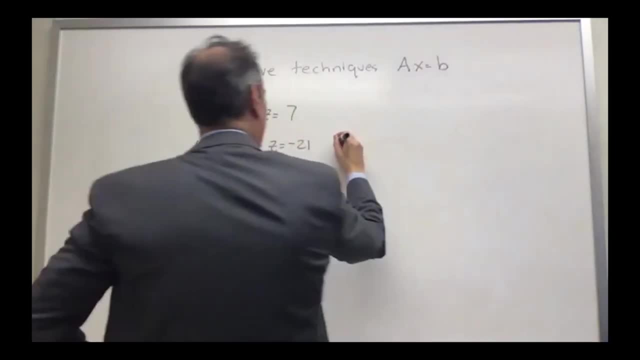 to solve for X. From the second equation, I'm going to solve for Y. For the third equation, I'm going to solve for Z. Okay, so what's going to happen here? From the first equation, solving for X, that means I'm going to solve for Y. From the second equation, I'm going to solve for Y. From the. 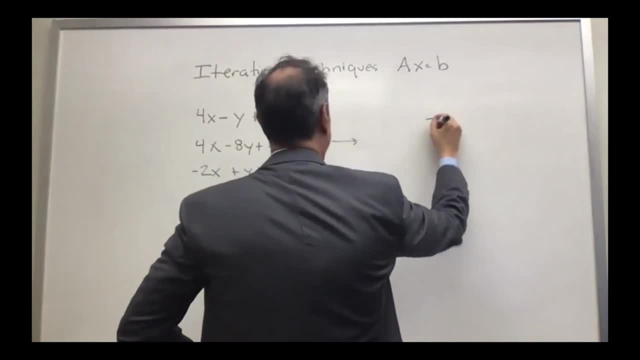 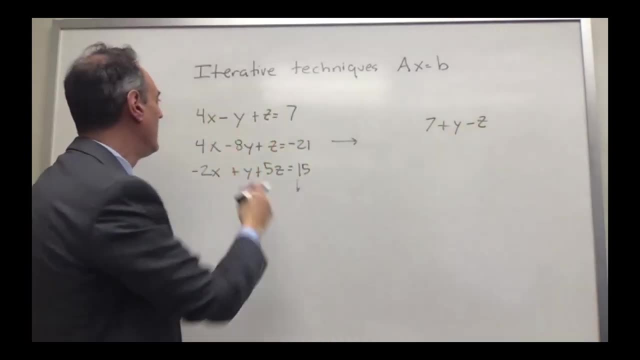 third equation I'm going to solve for Y. From the third equation I'm going to solve for Y. So I move the Y over and the Z over, So I get a 7 plus Y minus Z, right, And then I divide by 4.. 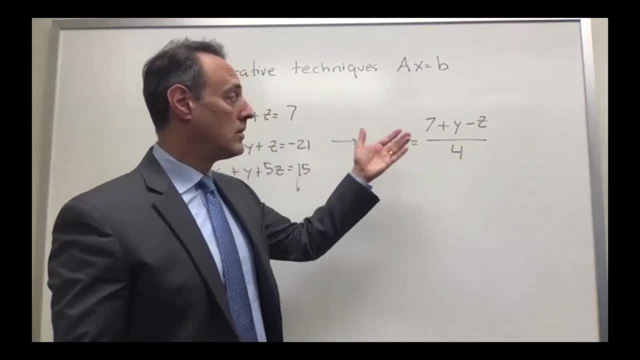 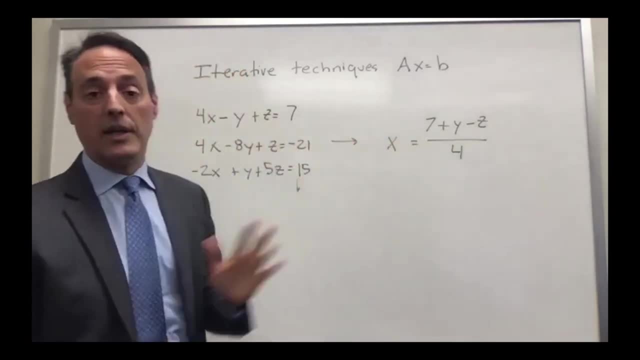 Now, of course, I don't know what Y is or Z or X, but here we go. I just rewrote that equation and I think we'd all agree that that works. I'm going to do the same thing for the other two equations, but the second one I'm going to solve. 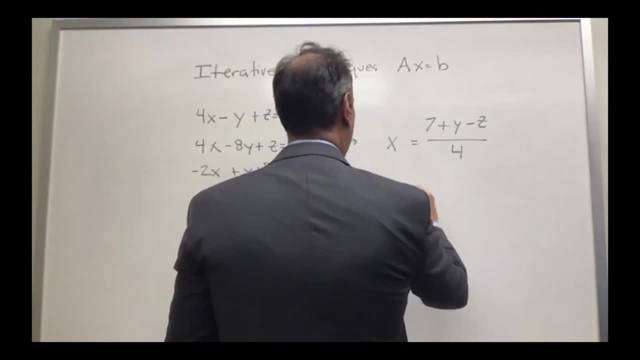 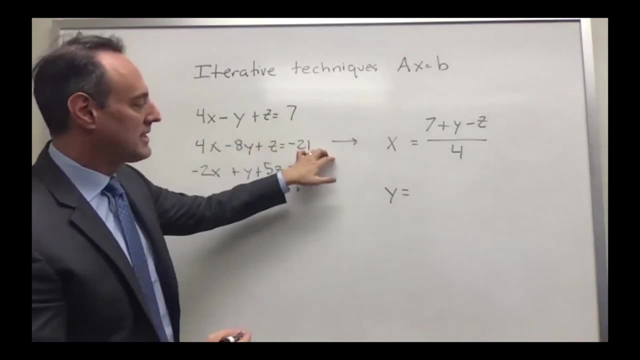 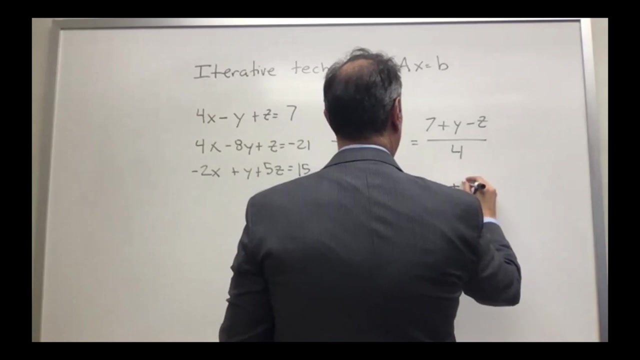 for y. Now, if I solve for y, notice I have a 21 over here. This is minus 8y, so I could make it plus 8y over here. move the 21 over becomes plus 21.. So it's 21 plus 4x plus z and all that's. 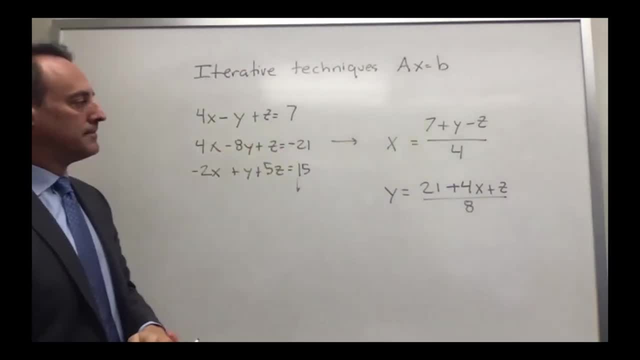 going to be divided by 8, which was in front of the y. I hope you're marveling at my algebraic skills. Hopefully I did it right Now for the third one, let's solve for z, So I'm going to. 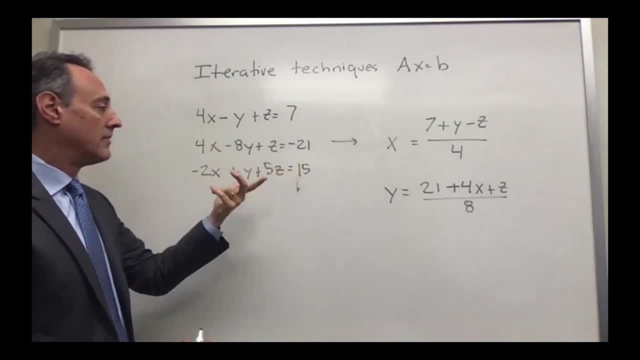 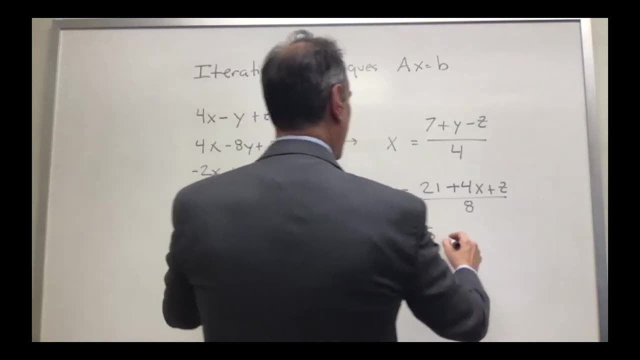 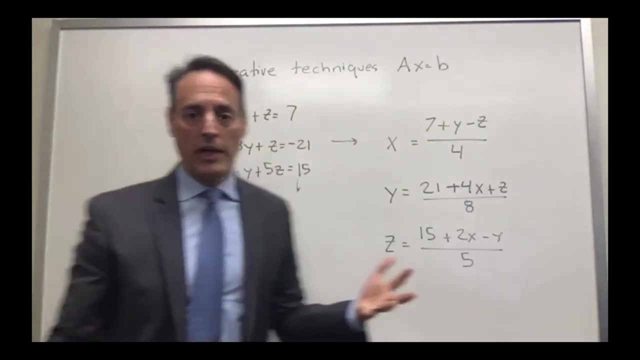 take this 2x over the y over and divide by 5.. So I'm going to have 15.. I'm going to move the x over here, the y over there, and I'm going to divide by 5.. So really, to some extent I've done nothing. I've just taken the 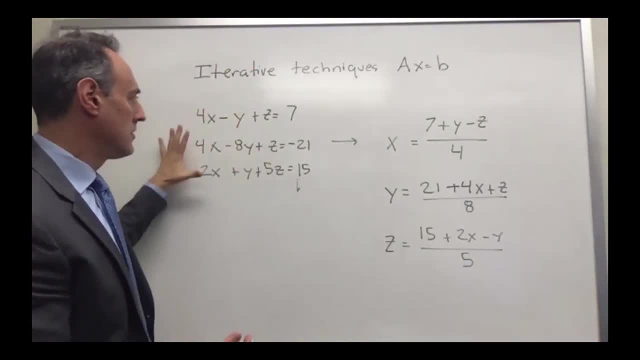 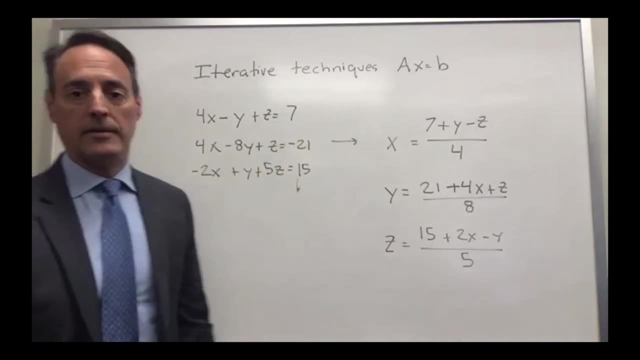 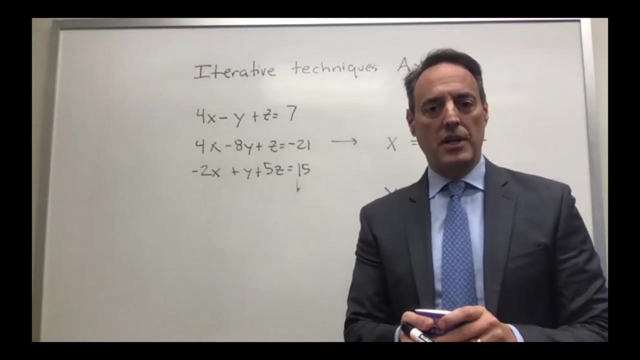 governing equations. three coupled equations here they are right, algebraic equations, and we're actually trying to solve for x, y and z, and all I did is I just rewrote them in this way. So there's nothing I've really done at all. And now here's where it gets kind of interesting. 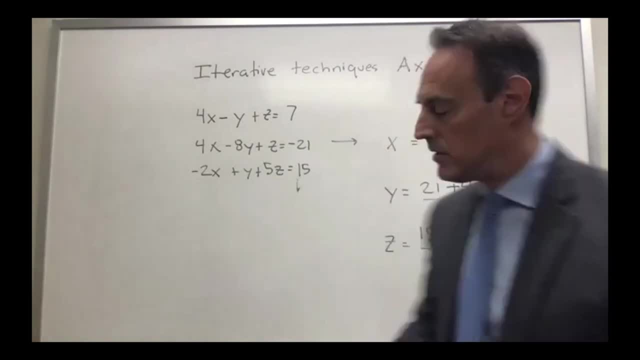 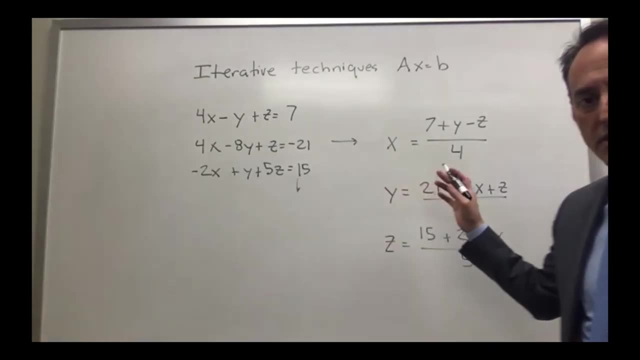 What we're going to do is we are going to take these and make an iteration scheme out of them. So what I'm going to do is take this here, and here's what I'm going to do with the iteration. I'm going to give you some initial guess. 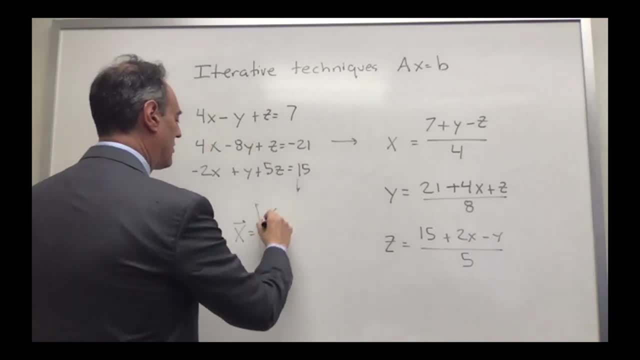 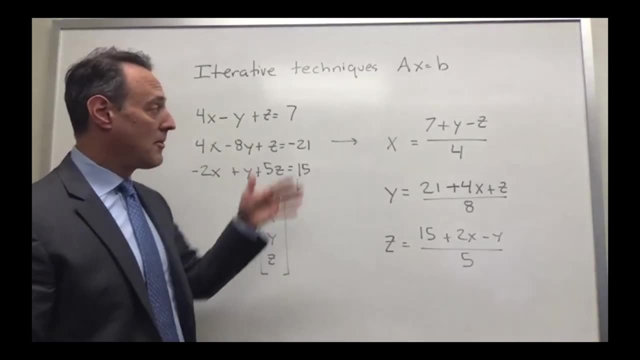 a vector which has initial values of x, y and z, And then what you're going to do is from those I'm going to make an iteration scheme here which is going to say my next value, x of m plus 1,. 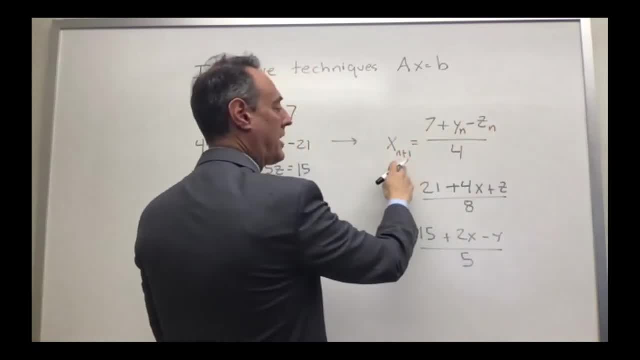 which is going to be the initial value of x, y and z, And then what you're going to do is from was the old values, and that's how I get my new value, y of n. then y of n plus 1 is equal to. 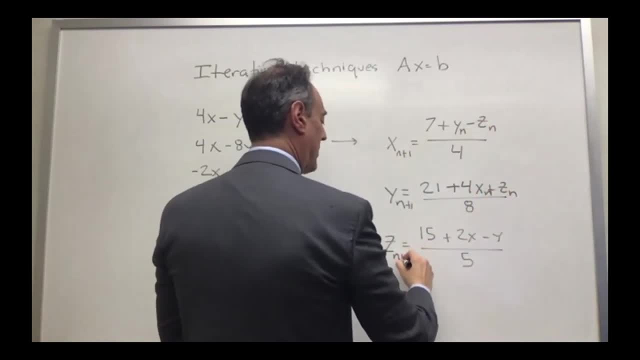 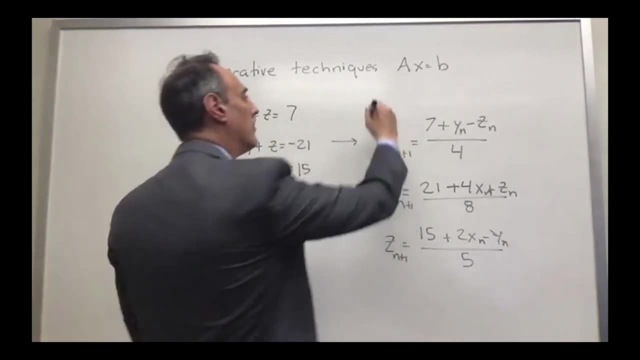 x of n. there, z of n and z of n plus 1 is equal to x of n, y of n. So all I did was said: if I give you, and then n equals 1,, 2,, 3, and so forth. I'm just going to put these in and iterate. 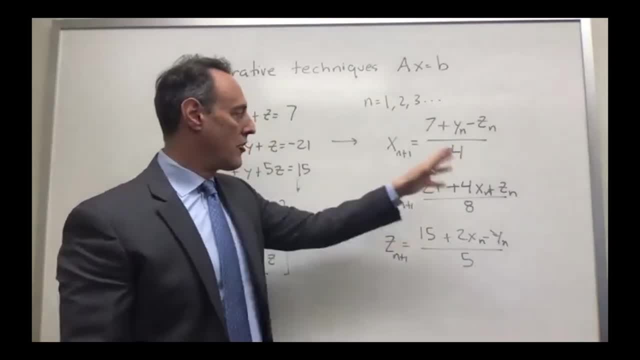 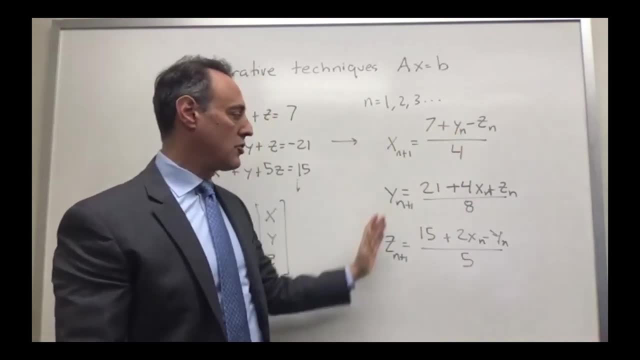 Get some values of x, y and z, throw them in here and when I guess these values, I put them in here as x1, y1, z1,. I get to x2, y2, z2.. Put those in here to get to x3, y3, z3, and so forth and just start iterating. 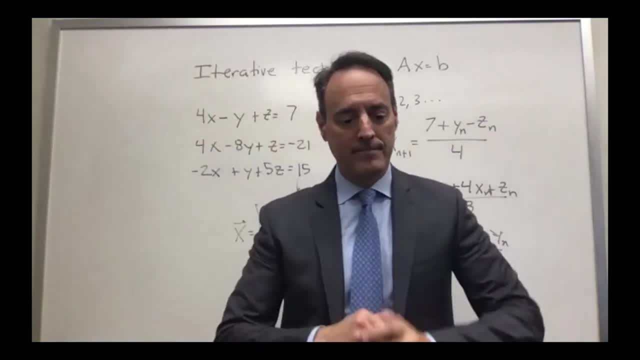 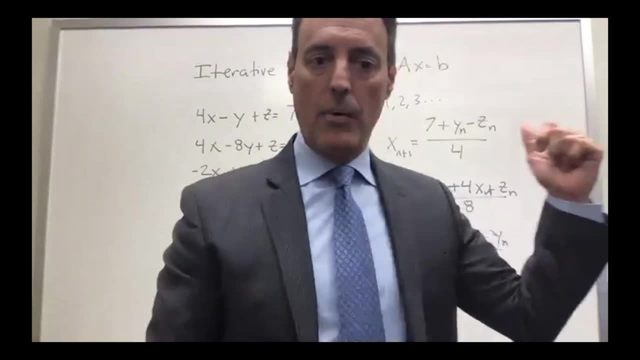 And then the question is: what happens when you do that? So let's write a code to see what happens. So what I'm going to do with you is share, do a screen share, and we're going to do exactly that. We're going to just iterate on this, this set of formulas here, to see what happens. 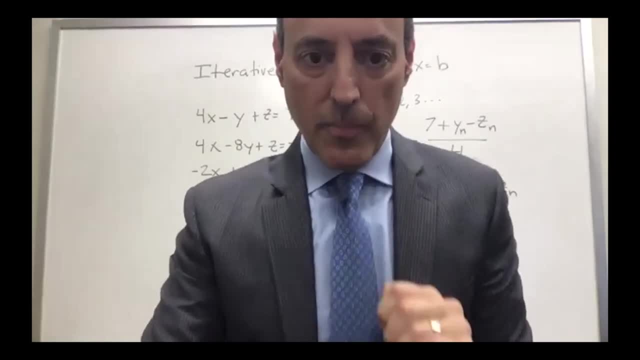 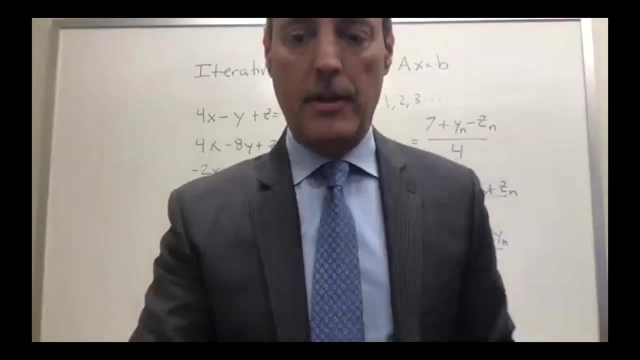 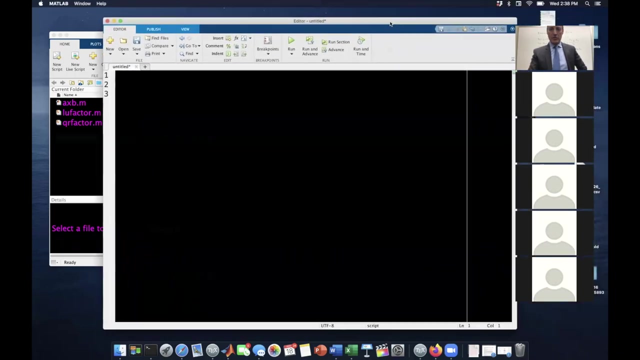 So let me go ahead and do a screen share here, and we're going to do my whole desktop. There we go, Share. Okay, All right, And let's put this down. Okay, There we go. Hopefully you guys can all see my screen here and we're going to just do a program Clear all. 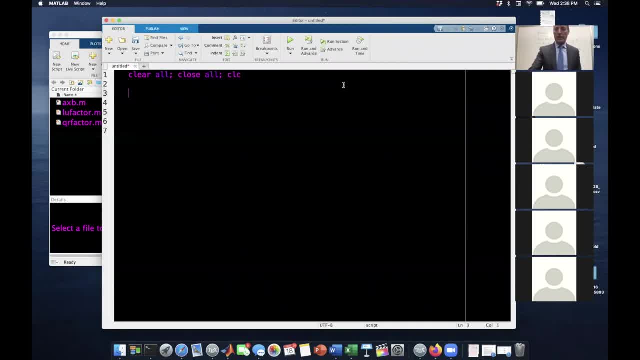 close all CLC, So that's always where I like to start my programs. So there we go. We cleared the whole slate and now we're going to do a program. So I'm going to do a program. I'm going to do a. 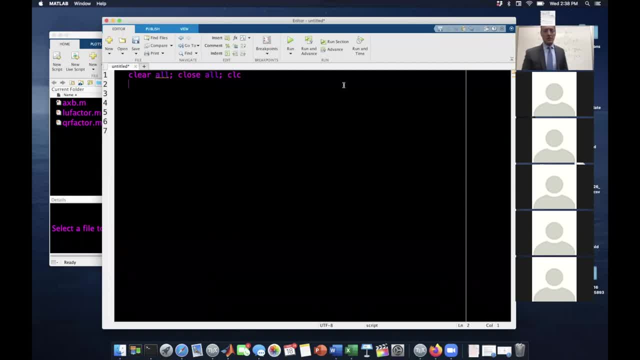 going to build this program which basically does this iteration procedure here. okay, so first of all, i have to guess some initial values, so let's keep- uh, let's keep track of this. there's a lot of different ways to do this, but let's just do. i have an x value initially. i don't know. guess 13, if you. 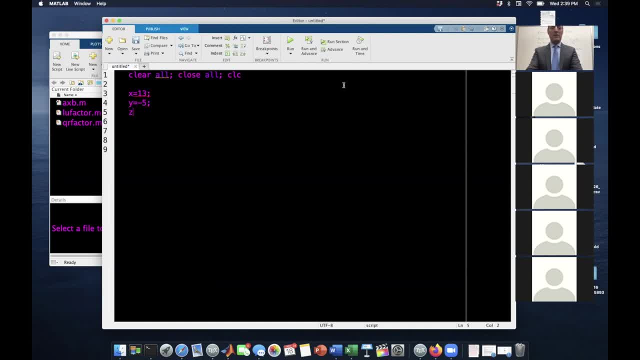 were in class, i'd make you guys guess what these numbers are, and i don't know. uh, pi. okay, there we go. those are my guesses for x, y and z. so i just start this off and, by the way, those are clearly not the solution. actually, i haven't told you what the solution is, but those are not it, and i just 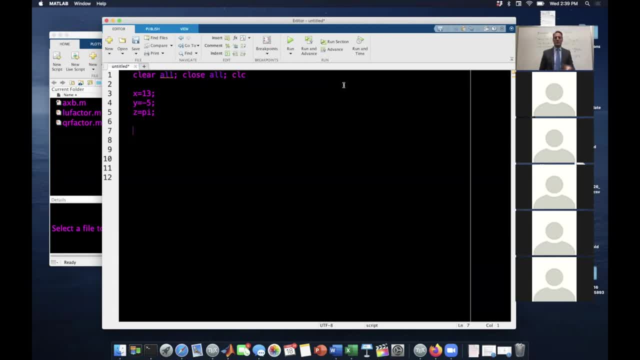 say: uh, i just give you some random values of x, y, z. you saw that, i just guessed it here in person. and what we're going to do now is we're going to just basically say, okay, let's go through this and let's go ahead. and in fact, you know, i'm going to make these vectors because i want to keep track. 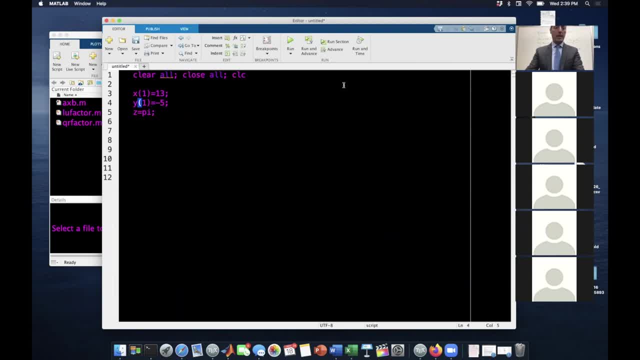 of them as we go along, as we iterate. i want to see what happens to these values. so the first value, x1, y2, and then now i'm going to say: do a loop, for j equals one, two, i don't know. let's do this loop 50 times there it. 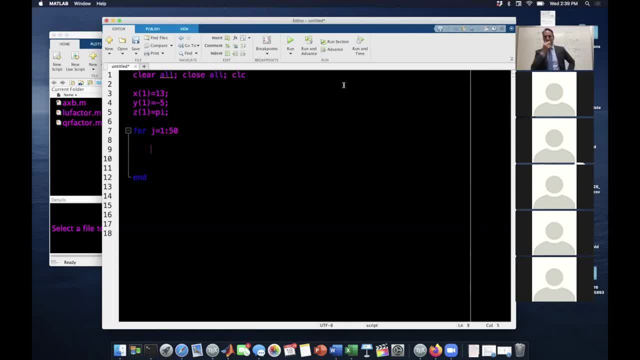 is sorry if the blue is a little bit light there, but that's what we're going to do. we're going to iterate 50 times doing this kind of structure here. and so what does it say? what it says here? then it says x of j plus one. 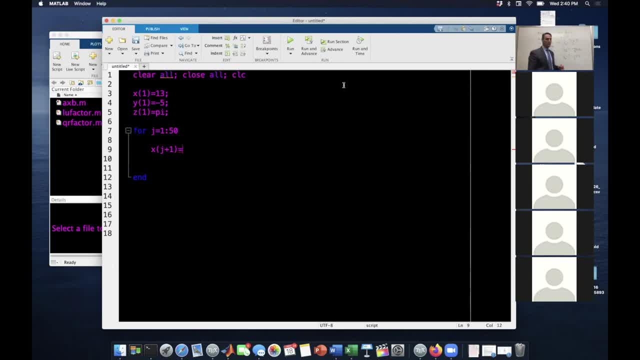 is equal to- and i have a formula up here and the formula says: i have seven plus y sub j, minus z sub j, all that's divided by four. okay, so that is the expression i derived from the first equation and when i moved everything over to this side, i got this expression for x as a function of y and z. 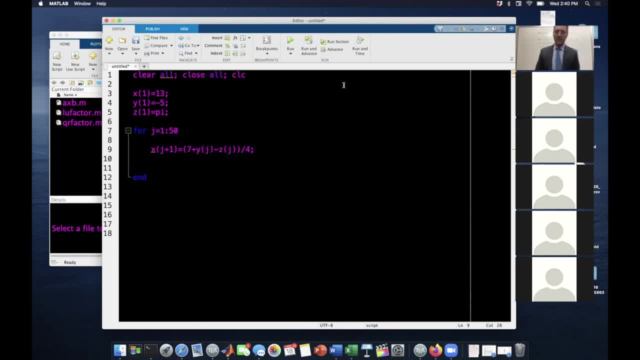 and there it is. so I'm just saying the next value of x is given by the previous values of y and z. all right, let's do the same thing for the y values and the y values. uh, they. I also had a formula up on the board. it's 21 plus 4xn plus z of n. so 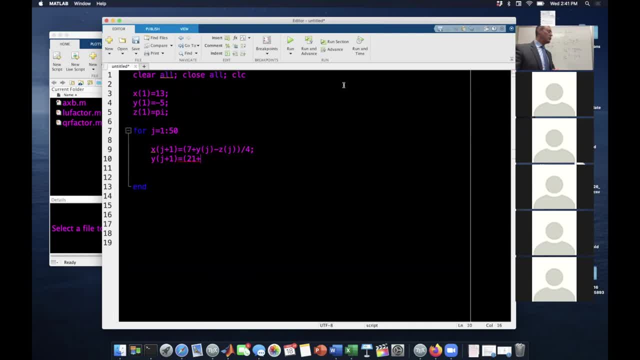 I'm going to put those in, and your job is to unmute yourself. if you see that I, if I have a typo in something here, okay, okay, all right, there we go. and then finally, the z of j is 15 plus 2 times x, j minus y of j. 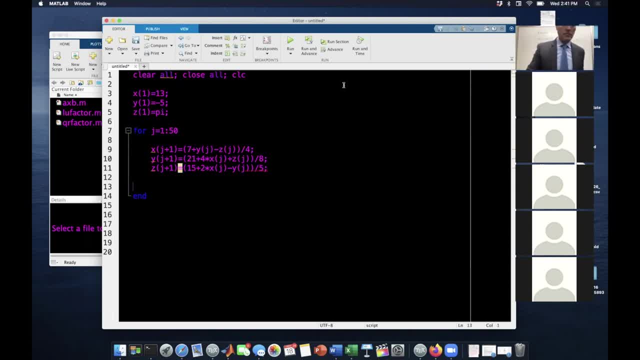 all divided by five. so there you go. that's my loop. I give you some initial guess. there they are, and I'm just going to throw it into this iteration scheme and what I'm going to get out is just a series of numbers, which is x, being updated from the previous values to the next value. 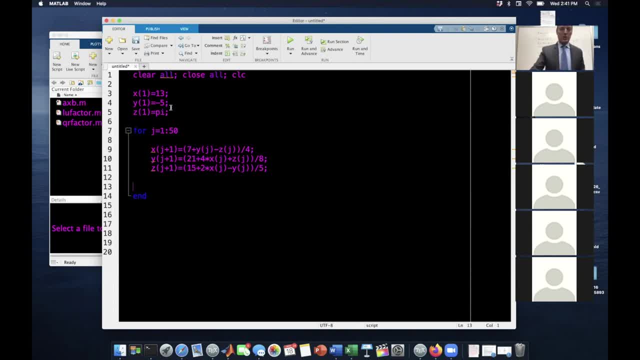 same thing for y and z. so we're going to do this loop and then at the end of this loop, like the amount of thing, I'm going to do this loop 30 times, I'm going to plot, oops, plot x. in fact, you know through this iteration, since I'm going to go 30 times. 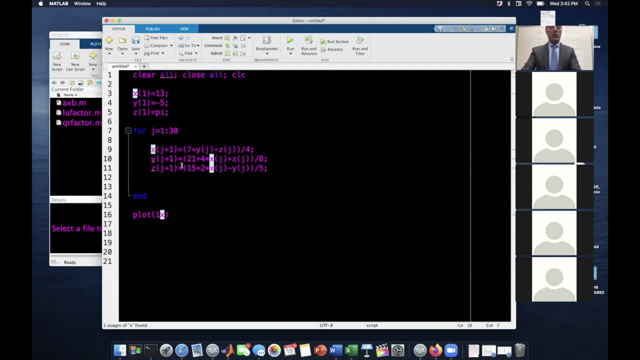 I'm going to end up with 31 values, right? so from 1 to 31, I will plot x. from 1 to 31, I'll plot y. from 1 to 31, I'll plot z, so they'd be in different colors, what happens with them? and in fact, let's plot these, uh, with balls because, remember, it's a. 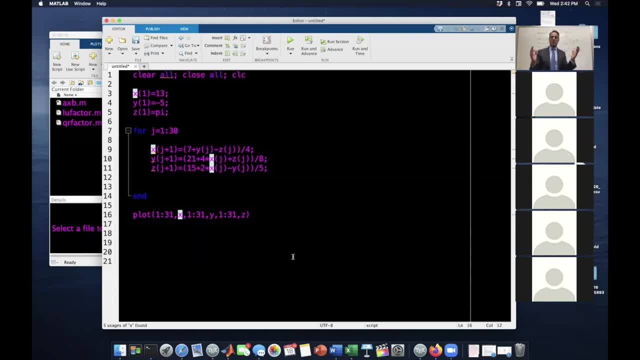 actually just see what it plots on its normal thing. okay, everybody, go with this. this is just a simple little code, just an iteration procedure. there's a couple things that computers are really good at. one of them is iterating. in fact, that's probably one of the best things it's good at. 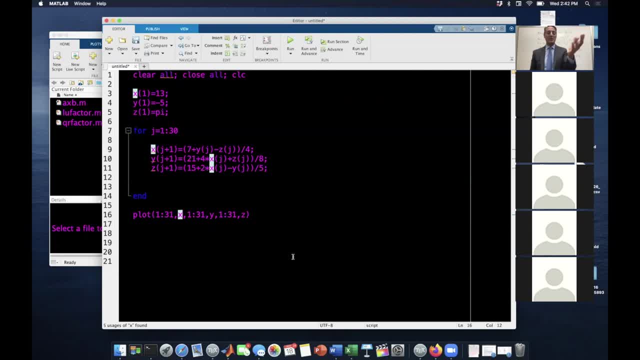 you're right that that's. that's what you normally use a computer for is iterations like this, because it'll just do that without complaining. and but you would probably complain if i made you do this loop 30 times in your head or write it down a piece of paper. 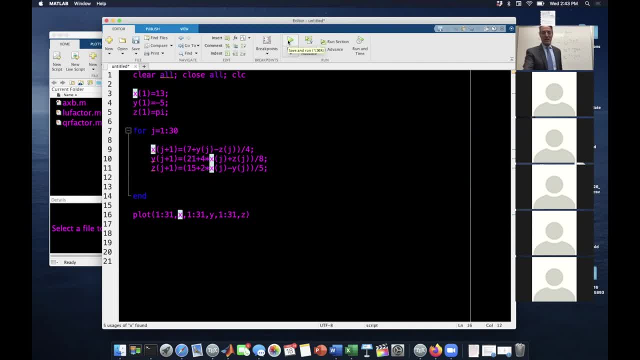 but not a computer, it'll just do it ready. let's run it, see what we get. oh, let's call this. uh, call this 584, demo, demo, 584.. save, it's running, done, and there are the values. and of course you can't see it because 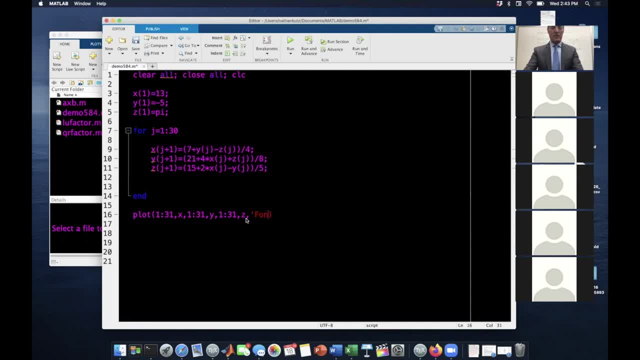 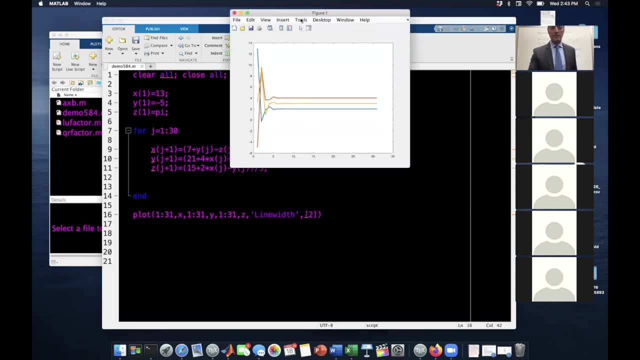 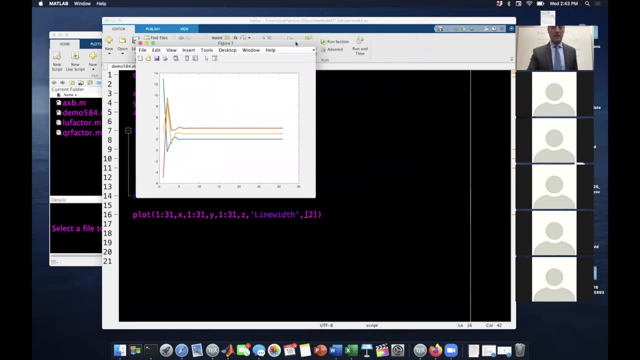 default settings are. actually i want to do a line width to let's run it again. all right, there's a little bit better. everybody see that, right, so i have to wait till let's blow this up a little bit. okay, so something interesting is happening here, so what? 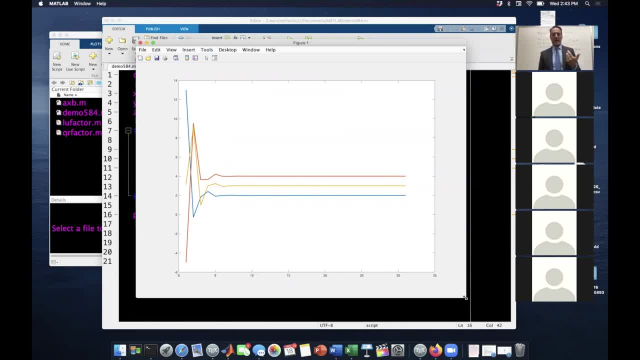 you're seeing, there is these three values of x, y and z, and as i iterate and what often happens in iterations, there's actually some very interesting things that happens in iterations. when you iterate things for a long time, uh, one thing that can happen is the iteration can converge. 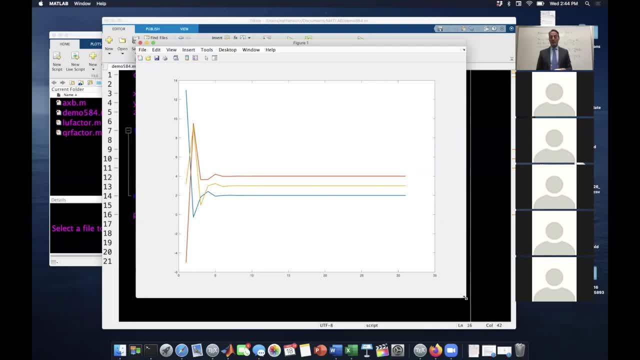 to some value, like it's doing here. another thing that can happen is it can blow up. another thing that can happen is when you iterate, you can get, you know, some chaotic mess out of the back end. there's a lot of things that can happen, but what's interesting here is notice it's actually converging. 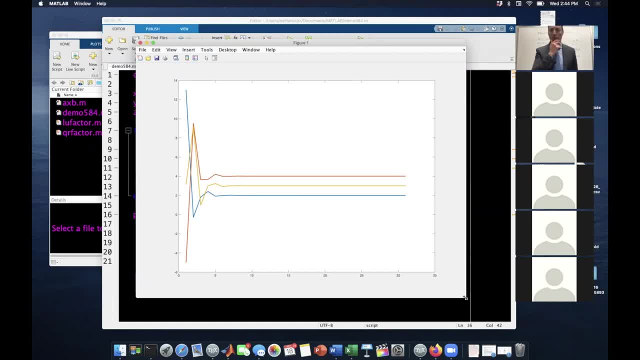 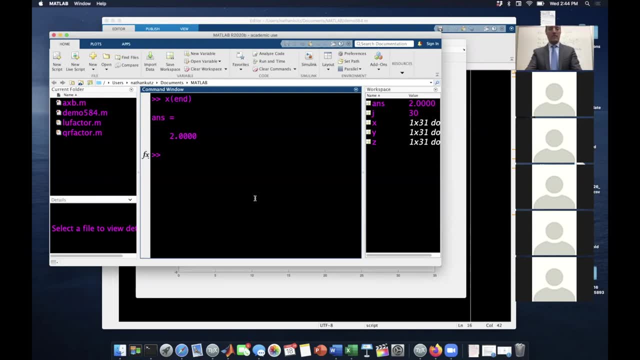 to some values and, of course, if we want to know what those values are, i can just simply come here to my terminal and say: what's the last value of x? it's two. what's the x value of y, four? what's the last value of z, three. so the last it's converging to two, four and three. 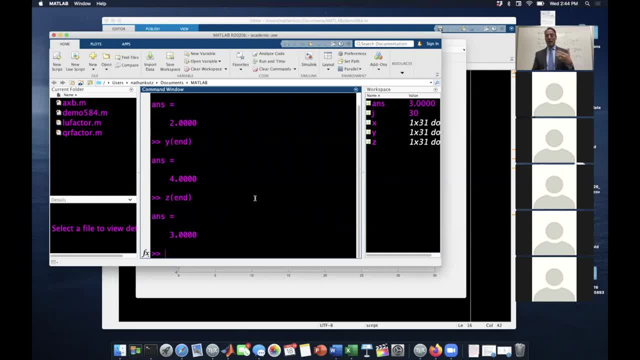 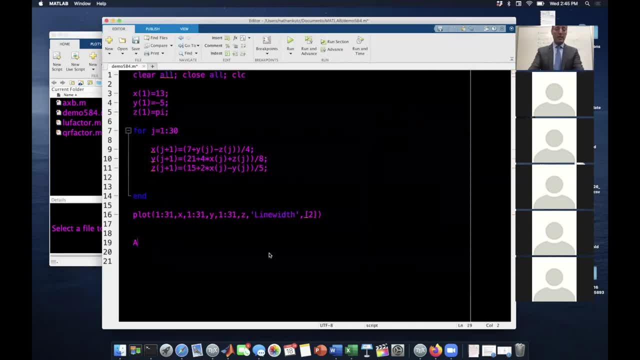 by the way, i could also ask the following question: what if i were to solve this problem? ax equal to b and in fact let's go ahead and do it. the matrix a in the system i had written down on the board earlier was four negative one one. that's the first row. second row is four negative. 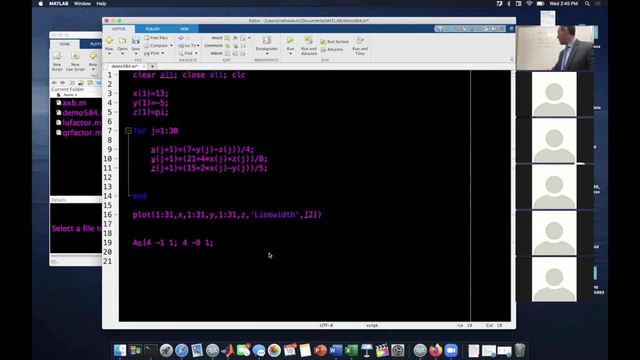 eight one. the third row is negative two, one and five, and b is equal to 7 negative 21 and 15.. and so the solution to this is: x is- or let's not call it, x is called. c is equal to a backslash b, and let's actually have it print out to the 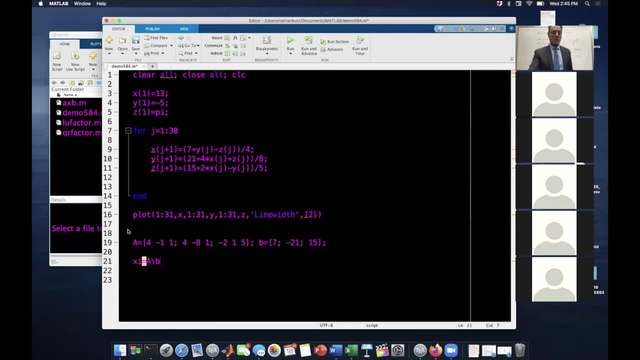 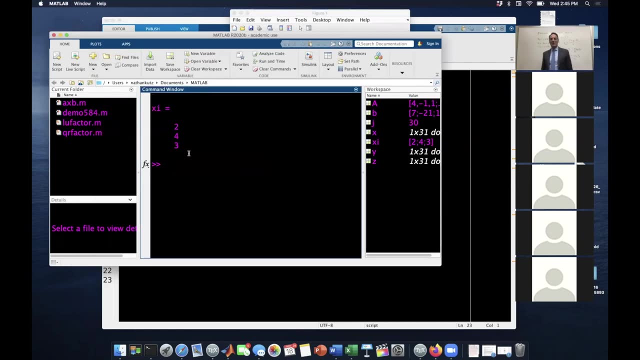 screen what these are. remember when this thing was iterating towards it iterated towards x was 2, was four, z was three, and when i just solve this, there is a solution and check out what c is: two, four and three. so when i did this iteration procedure, the iteration solved x equal to b for 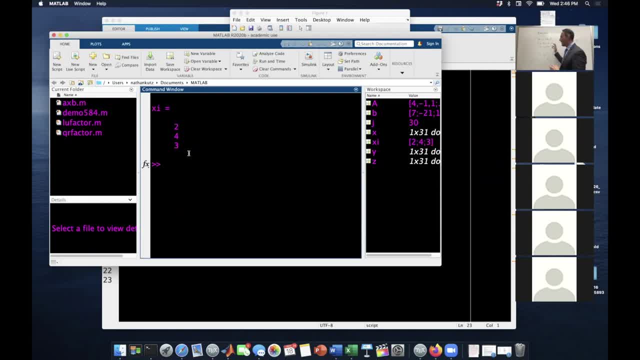 me. there was no dis deductive formulation here with lu, decomposition, gaussian elimination or something like this. all i did was took that governing set of equations, solve for x, y and z and look what happened. it totally worked. i actually got the solution out just by doing iteration. 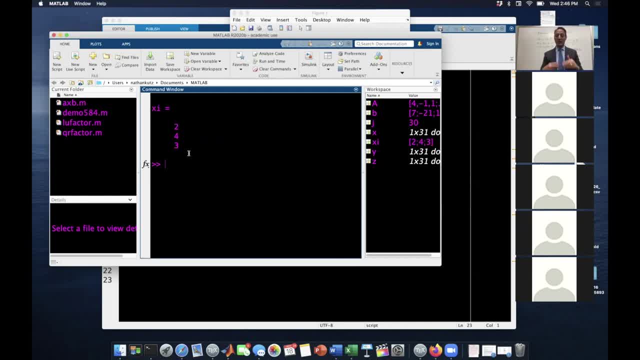 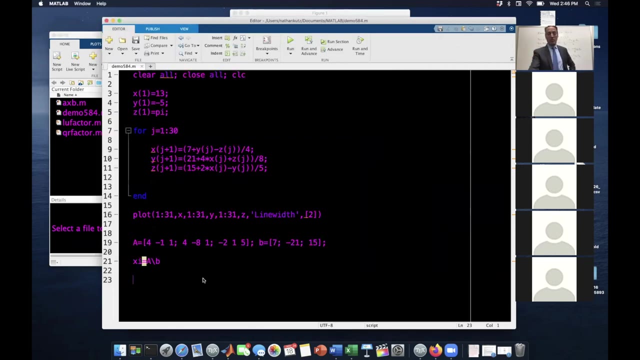 okay, so this is very interesting. this is starting to highlight something, a very different strategy for us computationally, which is, instead of a progressive set of algorithms that reduces x equal to b into some form where i can just solve for it. this is just simply. it seems to me, seems to you at this point, maybe that i just made up. 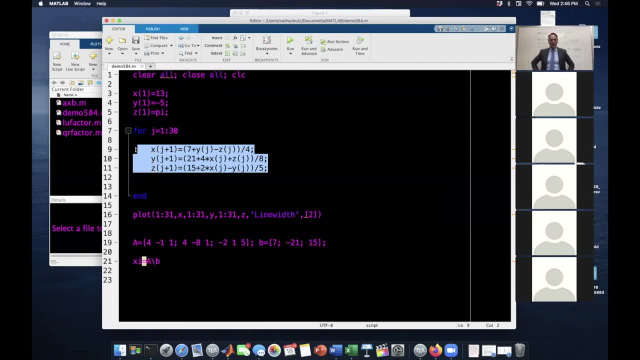 some iteration scheme, let it go, and the iteration itself produced this solution to this ax equal to b problem. so anyway, that's, i think, kind of remarkable, it's kind of an interesting property. and then the question is we're going to start asking: is huh, i wonder? 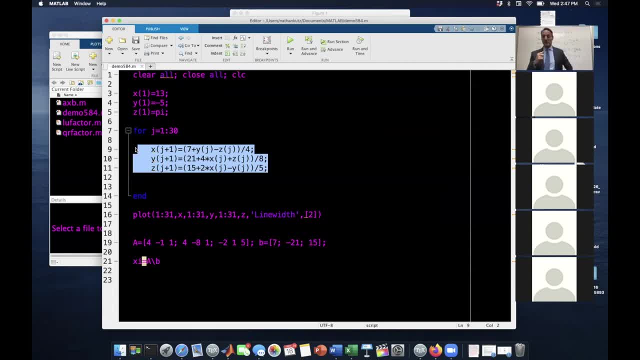 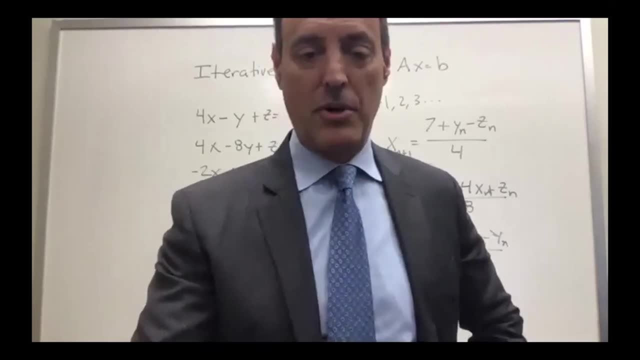 if this is, uh, maybe we should start thinking about what this means for us in terms of solving problems, because we're actually going to spend this week talking about solving ax equals b using iteration schemes, all right. so i'm going to stop sharing for a minute. we're going to come back to coding in a bit, all right, so 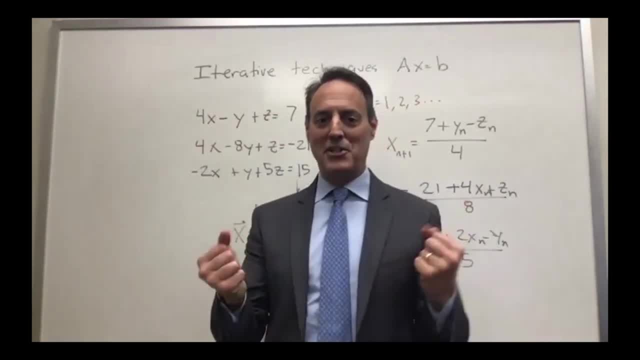 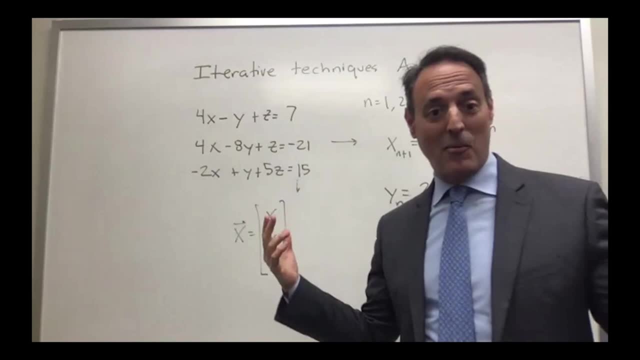 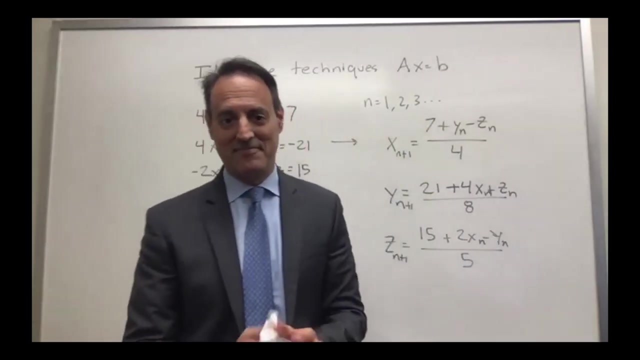 hopefully. that seemed like a little parlor trick, a little magic trick. look like you just take this equation, you just write it in a different way and you just set up an iteration scheme and boom, it works. how did that happen? let's try this trick again. okay, ready, we're going to do it again. you guys all saw what i did here. 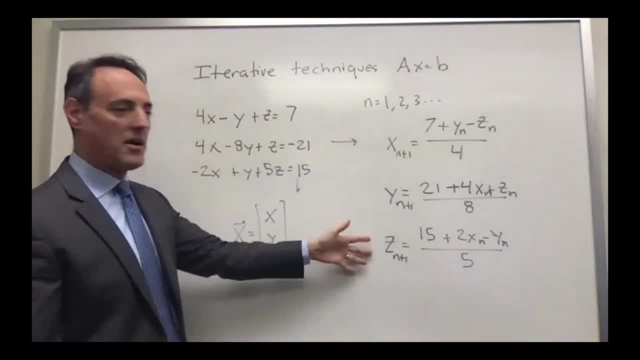 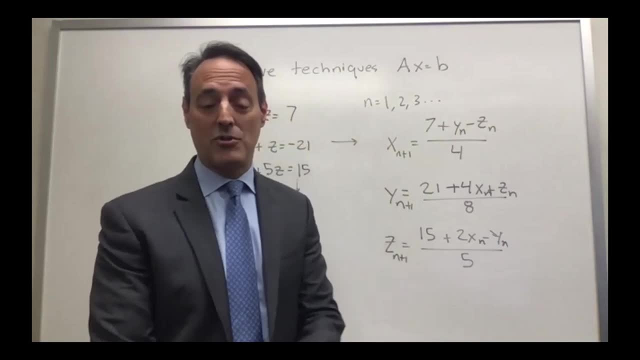 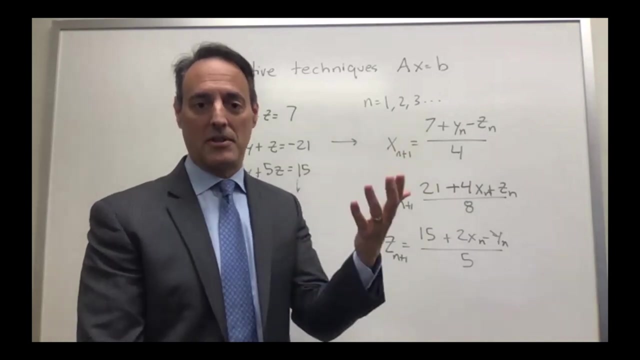 from these three equations i saw for x, y and z. there they were, set up an iteration scheme, just let that thing go and the resulting values. in fact it converged within like, if you notice, i went 30 iterations but pretty much it had been converging within like probably 10 iterations. that got me the. 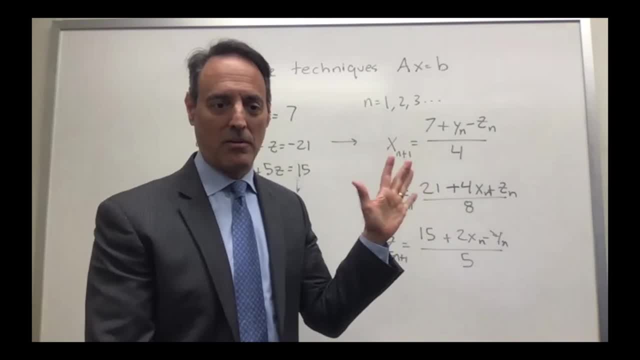 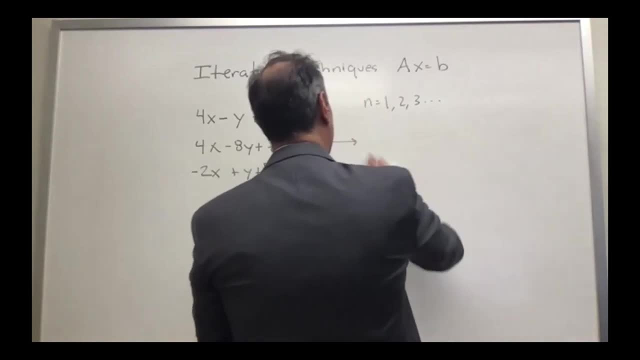 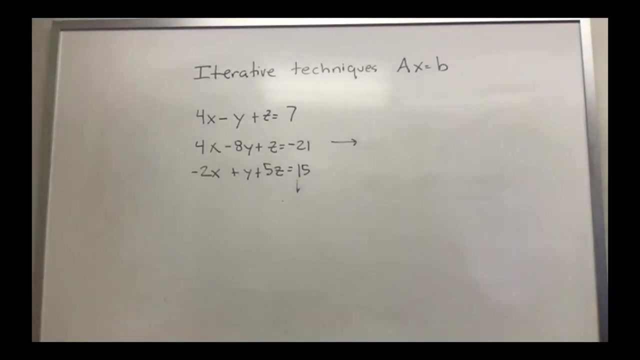 solution. okay, so let's come back to this problem and let's do one thing. i'm going to take this again and we're going to work on it, and what we're going to do is we're going to rewrite these equations specifically. i'm going to ask you: 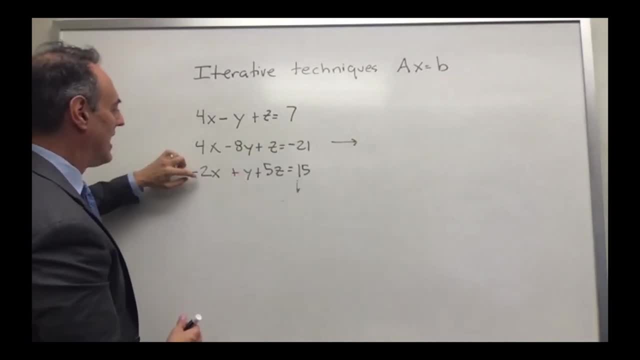 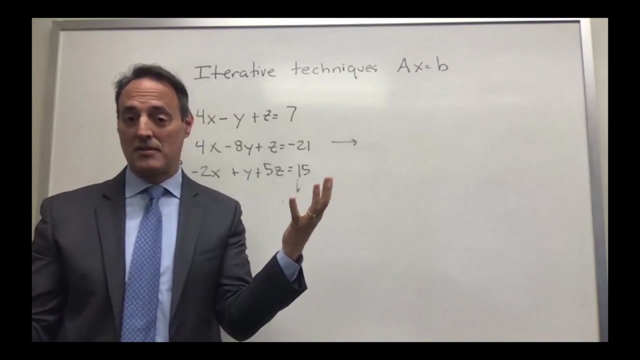 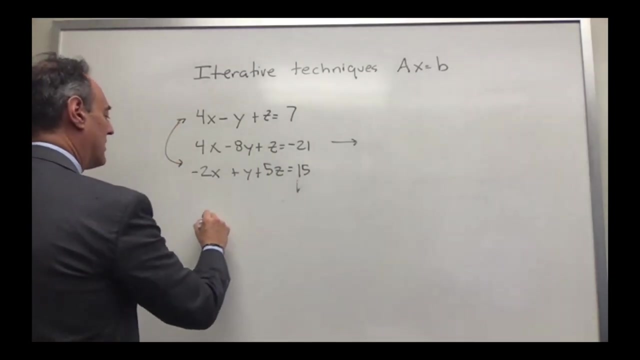 the question. if i were to take this row and switch it with this row, you would agree. i think that. well, i didn't do anything right. i just switched two rows. they're still the same governing equations, the same three by three system of equations, right? so i just switched them. so, in other words, i could write this as negative: two x. 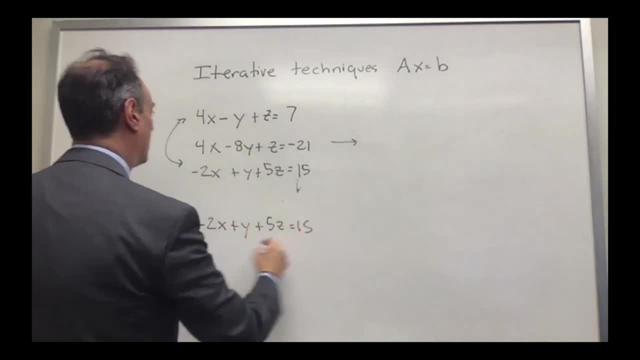 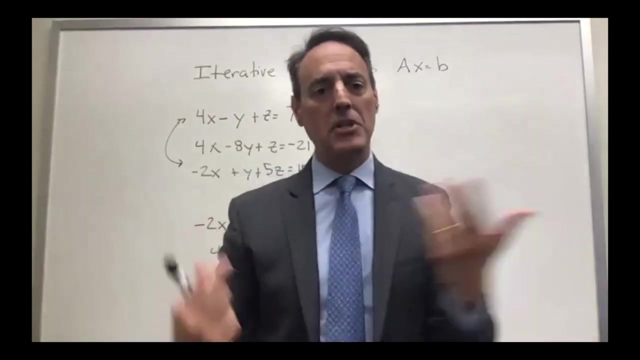 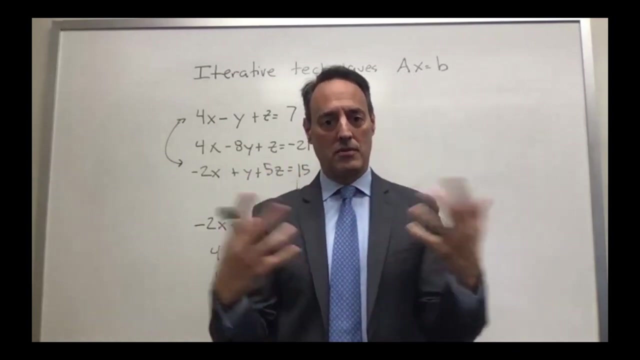 plus y plus five z equals 15.. four x minus eight, y plus z equals negative 21. and then here, four x minus y plus z is equal to seven. in fact, when we did the lud composition or gallop's elimination, remember that we always had to keep track of whether we're going to switch rows right, because we know we can just switch rows. 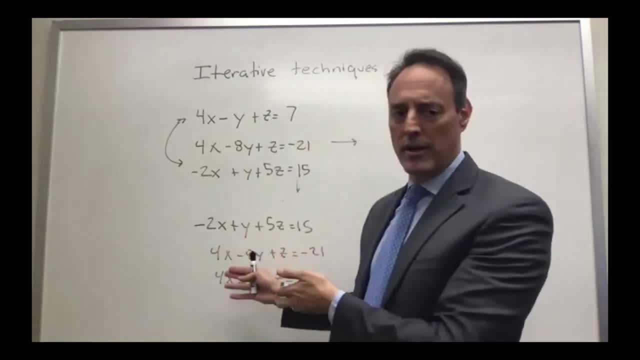 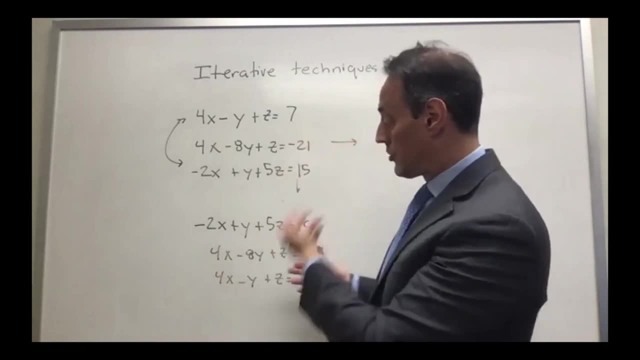 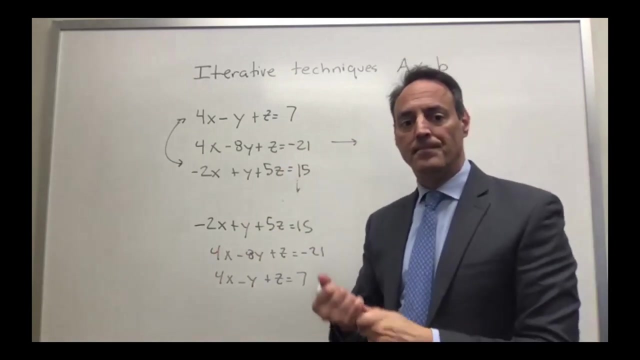 they're the same governing equation. so switching rows. all you were trying to do is avoid a zero pivot, and so you could do that by switching rows. and so i did switch rows in the same governing solution- four, three, two right- which is we had on a computer there. all right, but let's try this trick. 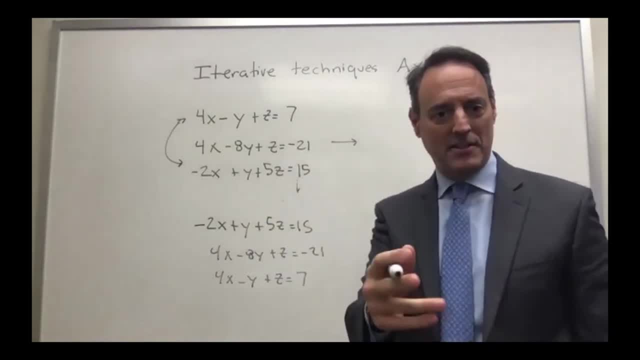 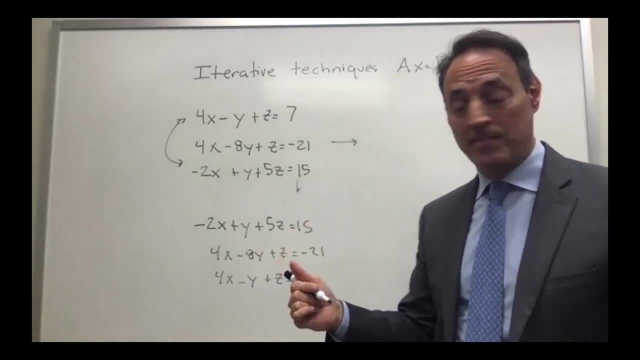 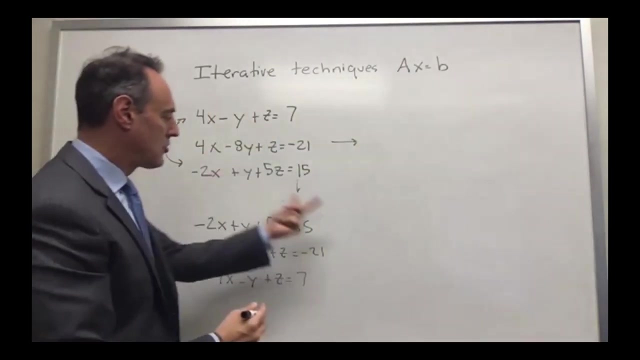 again now. from the first equation, solve for x. from the second equation, solve for y. from the third equation, solve for z. then make an iteration scheme. okay, so from the first equation now i'm solving for x. so this is minus two x. so i'm going to take the minus two. i'm going to take the minus 2x. 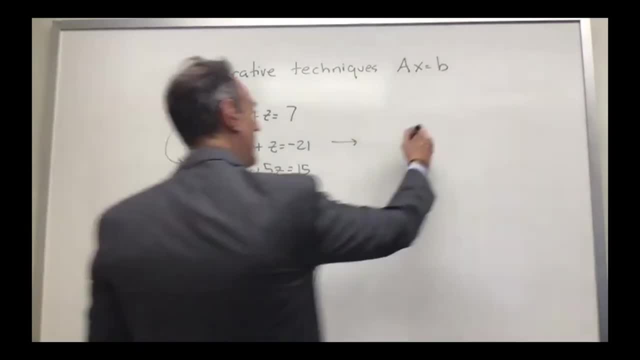 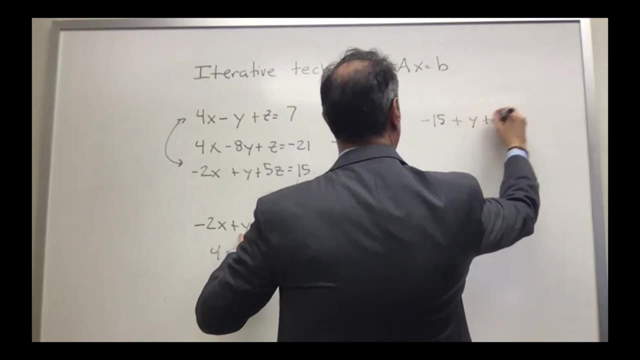 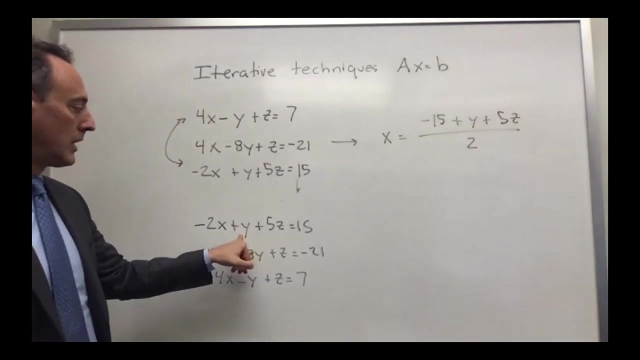 over here will be plus 2x, being the 15 over. so it's going to be minus 15 plus y plus 5z, all divided by 2. okay, so the minus 15 that comes over is 2x divided by 2. that's what you get from the second. 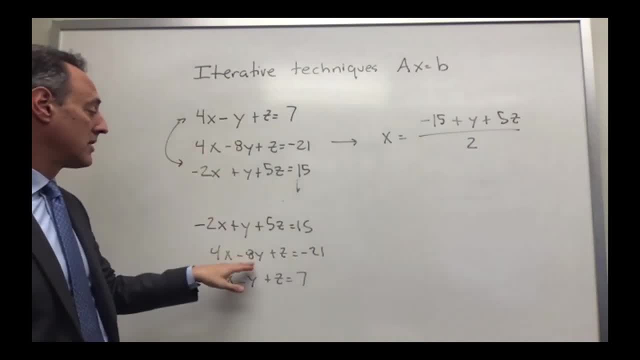 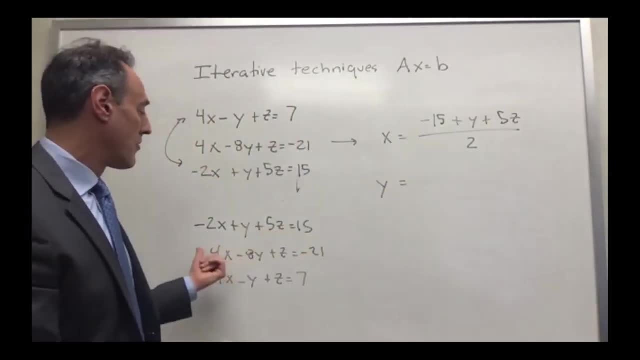 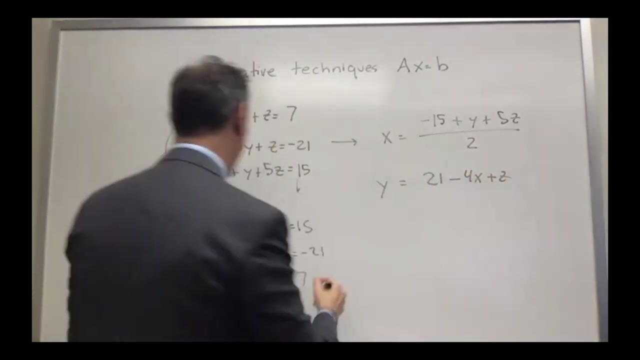 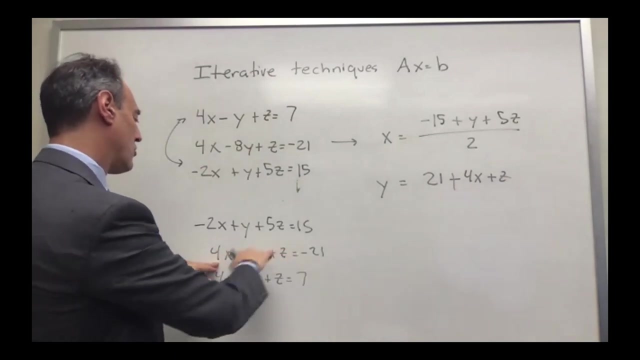 equation, i get exactly what i had before, so i should have just not erased it and kept it. but fine, y is equal to, so i move the 8y over here, the 21 over there. so i have 21 minus 4x plus z. sorry, i, i brought that over here. so it's plus 4x, right? so 4x z the 21 comes. 8 comes over here. 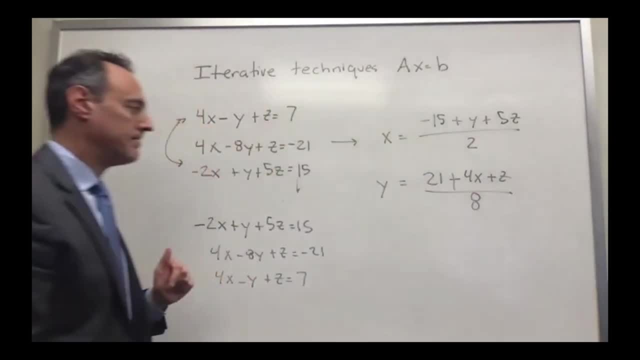 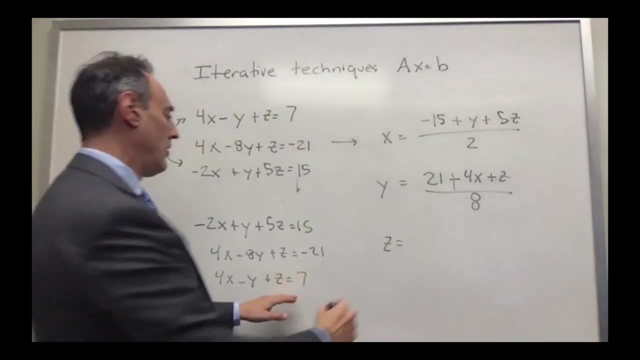 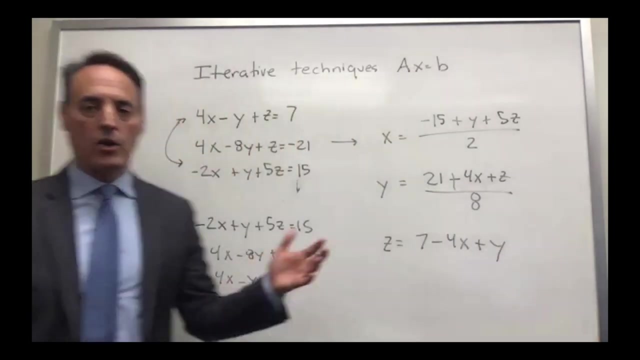 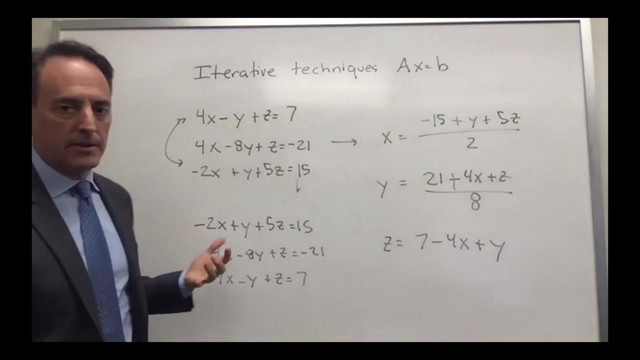 so there's a divide by 8. finally, from the third one, z was equal to. i can just move everything over. you have 7 minus 4x plus y. everybody agreed that. i just i mean look all we did. from here i solve for xyz. i just change rows. from here i solve for xyz. 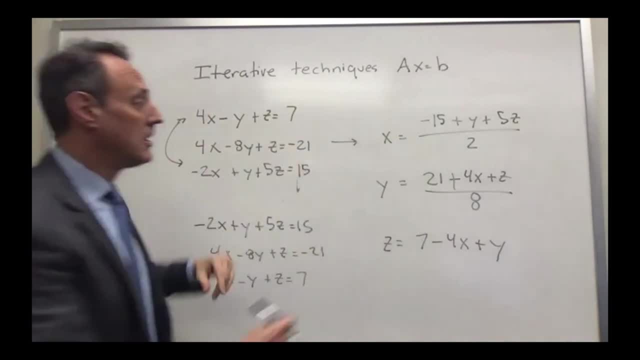 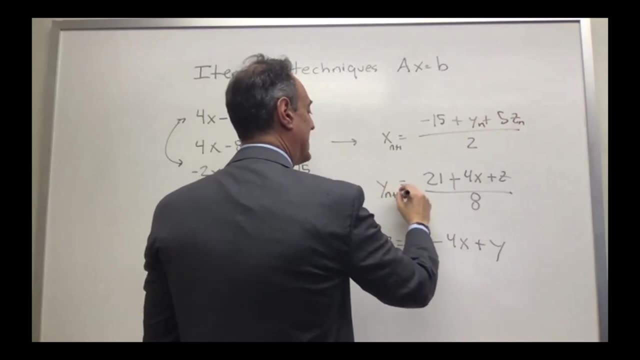 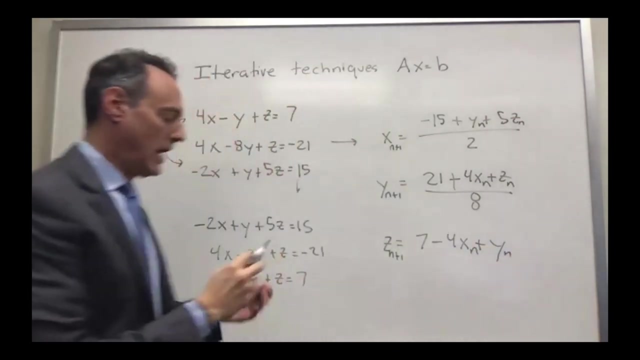 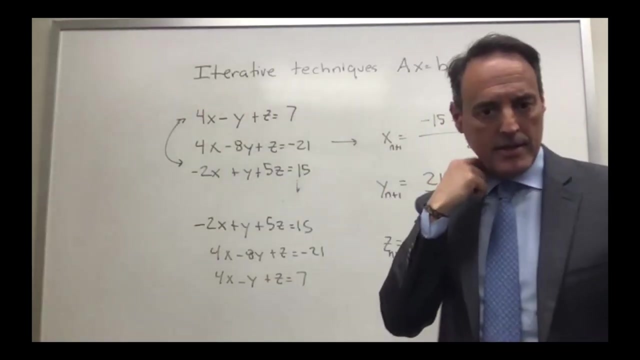 i get a different iteration scheme now, notice, because now i have: x of n plus 1 is equal to this equation, y of n plus 1 is exactly what i had before, and z of n plus 1 is this here. okay, so a slightly different iteration scheme. 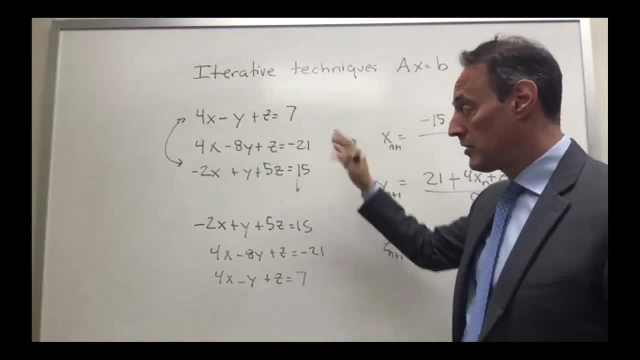 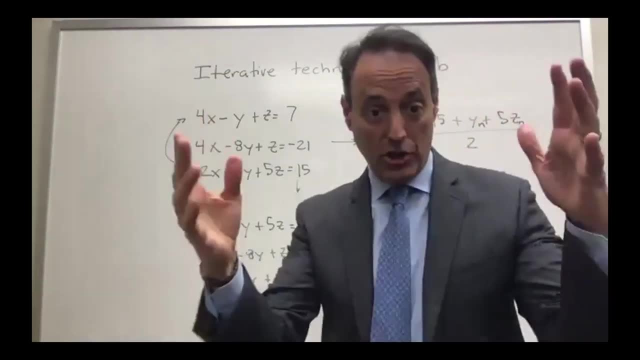 same set of equations, so really same solution, just interchanged rows, different iteration scheme. but let's go to it. let's go try to do this, because it should work right. you should get the same solution, uh, as before, because of course the solution didn't change it's. 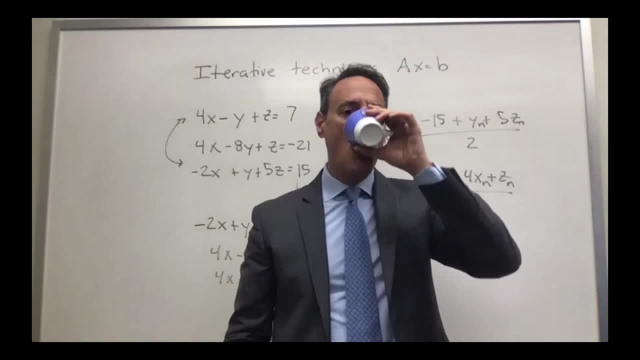 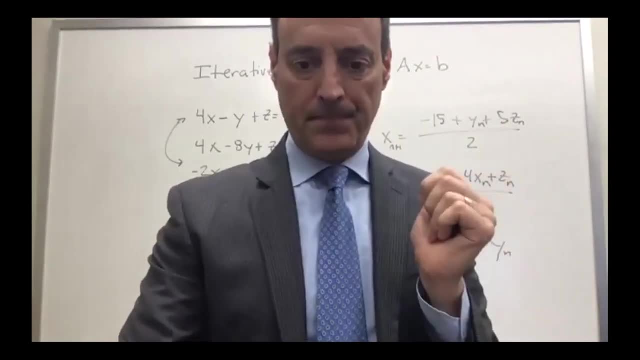 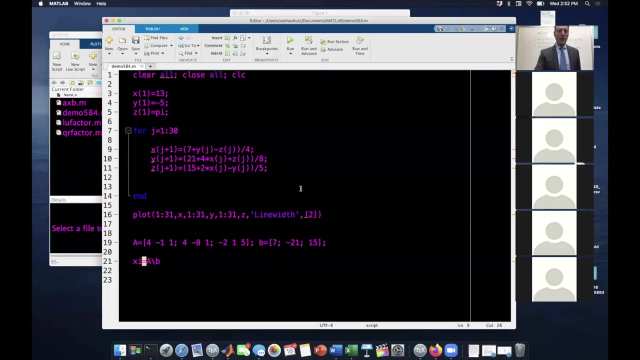 still four, three, four, two. okay, so let's go ahead and set up an iteration scheme to do this. so i'm going to go back to screen share. uh, share the desktop, boom. there we go, i'm back here. so we're going to keep this right. this is our method one for doing it. we're going to start off with the. 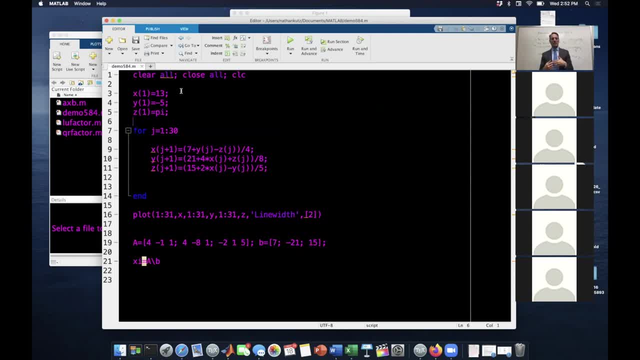 same guess. uh, let's let's go ahead and start off the same guess. but now what i'm going to do is, let me just say that, uh, let's run two iteration schemes simultaneously, so, like i'm going to make x2, 1 is equal to x1, so i'm going to, in other words, i'm going to have two solutions. 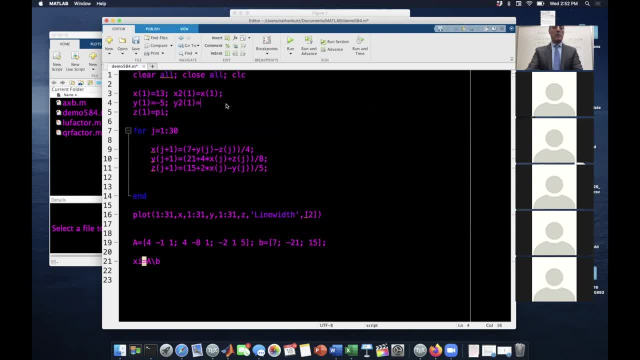 x and x2 and y2, which is, and what i'm going to do is compare these. how do they look relative to each other? because, in fact, they're solving the same system of equations, but they have two different iteration schemes. so i'm going to start off. i have this loop that's going to: 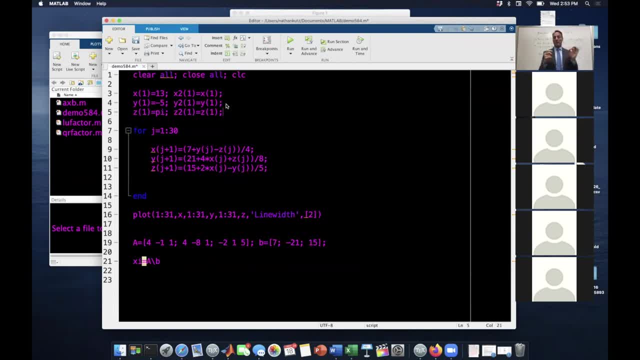 solve for xyz and i have another. i'm going to have the same loop and evaluate what's happening to x2, y2 and z2. okay, but now what does x2, y2, z2 look like? well, that's this new iteration scheme that i just wrote up on the board, so let's go ahead and 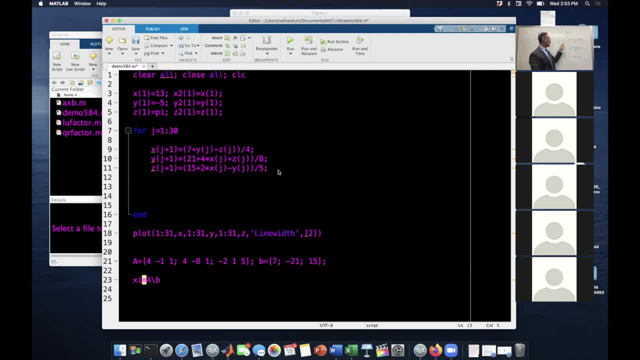 program this in, so you see that x of n plus 1 is minus 15 plus y of n, z of n. so you're going to get x of 2, j plus 1 is equal to. you have minus 15 plus y sub 2, j right, plus five times z sub j. 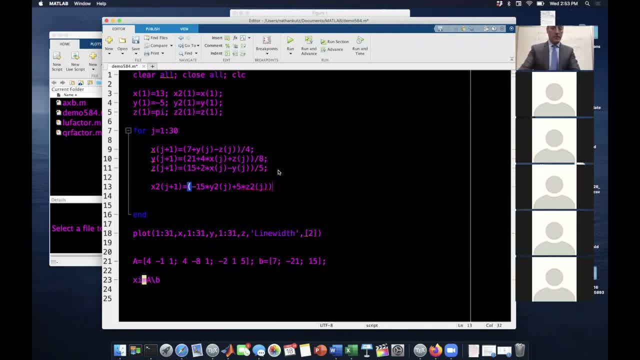 z, sorry, z2 sub j, okay, all divided by 2, and then you have y of 2, j plus 1 is equal to 21, plus four times x of n. four times x, that's what you get there. four times x2- now, because we're working with that- plus z2 of j, all divided by eight. now, this equation is exactly what i had. 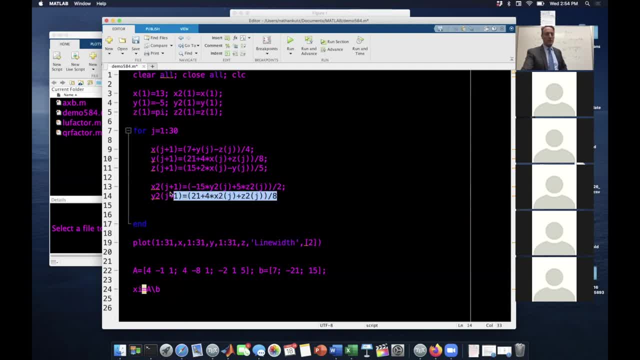 before. okay, so nothing changed with that equation right there, because i only switched the first, two and third row. and finally, z2 j plus one is equal to what i have up. there is seven minus four times x2 j plus y2 j. all right, let's put some semicolons in there, so i don't see all the output. 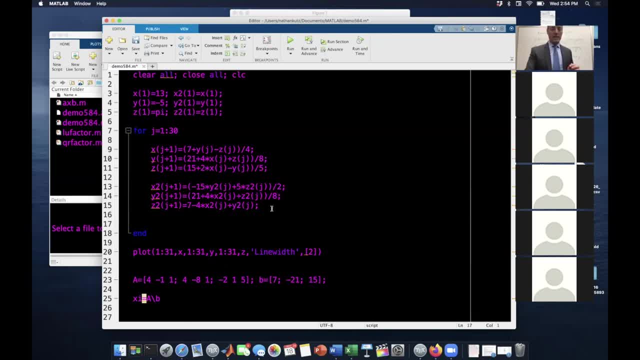 hopefully everybody agrees that this should produce the equivalent solution. is that, hopefully that's the case? that's what we want to check. is like somehow that iteration- if you've never seen this before- hopefully you're like: oh my gosh, you could just do that and iterate and it gets the solution. that seems magical kind of kind. 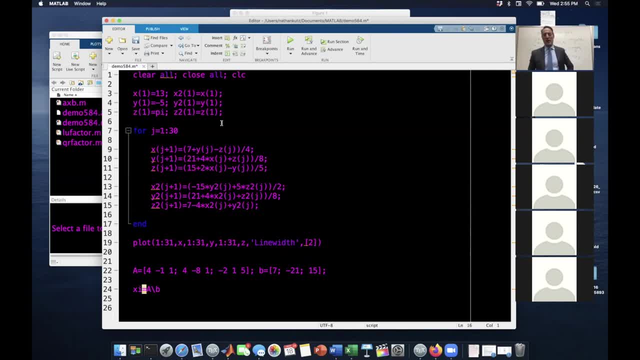 of pretty cool, right? um, and hopefully that's your thought, and if you've seen it before then, then this is uh, well, whatever, maybe it's a boring lecture for you, but okay, we're still going through this to see what these are. so now what i'm going to do. i'm going to make a new plot, so i have figure one. 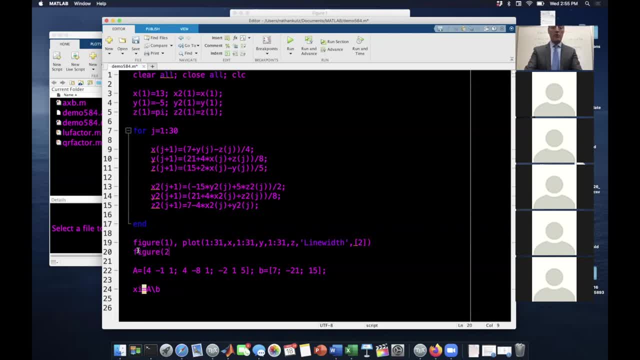 which will be the plot of the original iteration. i'm going to make a new figure, two, which will be this plot here, which is going to be basically same thing, but now i'm going to plot 30 iterations of x2 versus y2 versus z2, so two figures, and i'm going to say, just go and see what happens here, like i'm feeling like i'm going to be able to do this and i'm going to be able to do this and i'm going to do this and i'm going to be able to do this and i'm going to be able to do this and i'm going to. 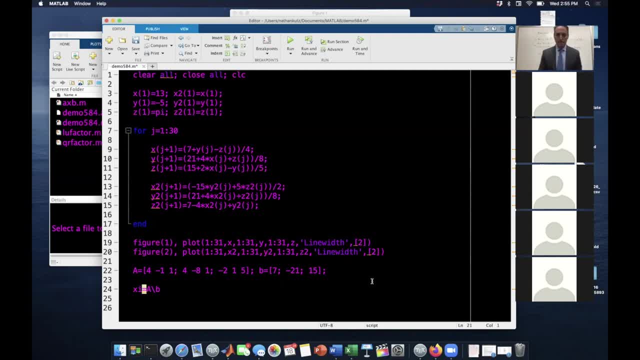 lucky this iteration. professor, i think you might have a typo on x2. i think it should be: uh, negative 15 plus y2j. oh, yeah, right here. yeah, is that? uh, yes, thank you. yes, yes, any other typos, thank you? i always like to get the typos before i hit return, i mean usually. 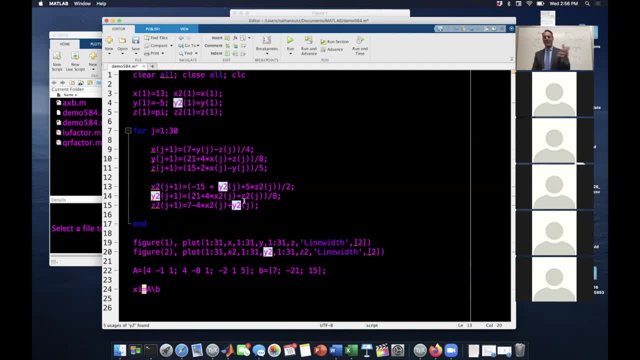 in matlab i'm always like it complains because i did something wrong. but every once in a while i'm you got on a hot streak where it always works every time you hit. go all right, thank you all. right now i think we're ready to plot these. hopefully, everything's fixed, all right, so let's. 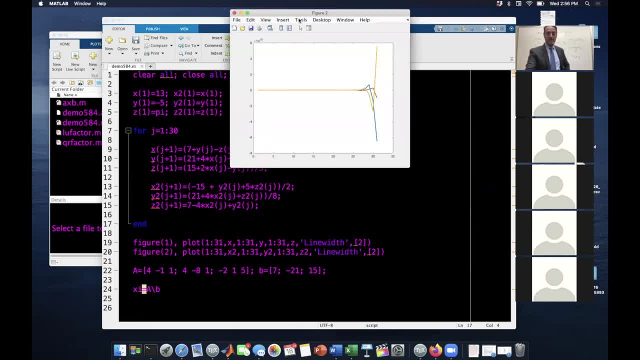 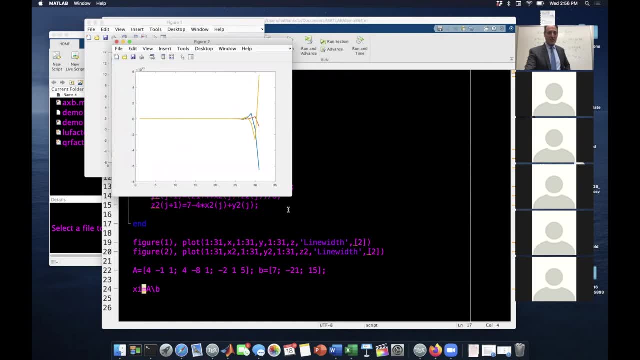 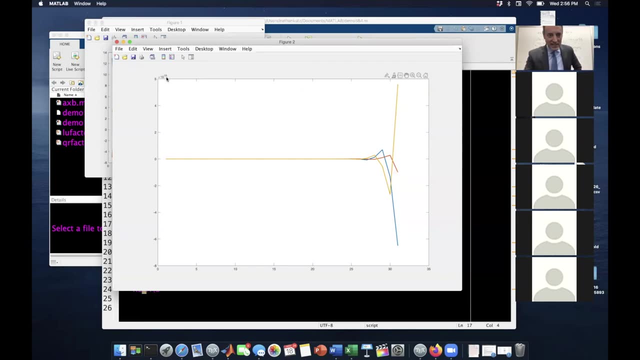 see what happens, run. oh okay. so here's what happened before and here's what's happening now. so you say what's happening. and, by the way, do you see this number right there? i don't know if you can see it. It says times 10 to the 15.. 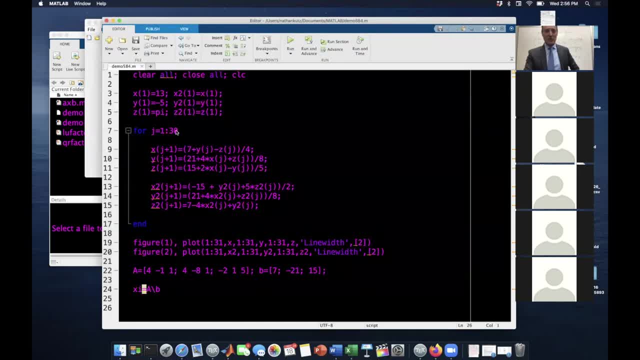 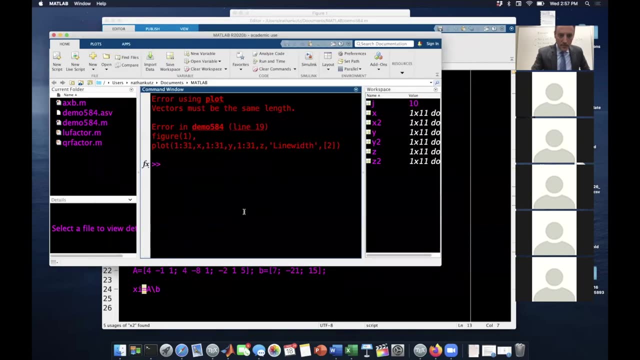 So what's happening is, in fact: let's go through a smaller number of iterations. Let's just go through 15 iterations. Sorry, Let's go through 10 iterations. What happened? Oh, I see I have to change these now. 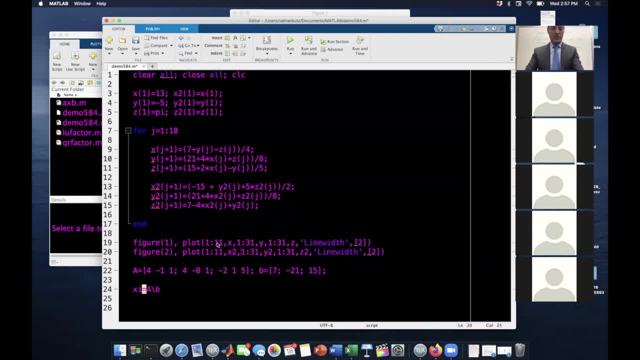 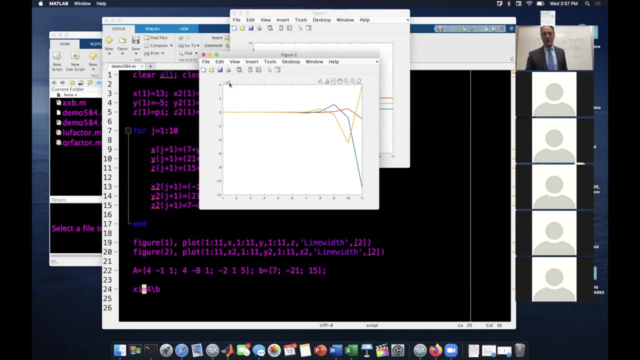 If I only do 10 iterations, I've got to change these to 11. now, OK, run it And there you go. And by the way, it already says 10 to the 5.. So what's happening? I told you earlier. 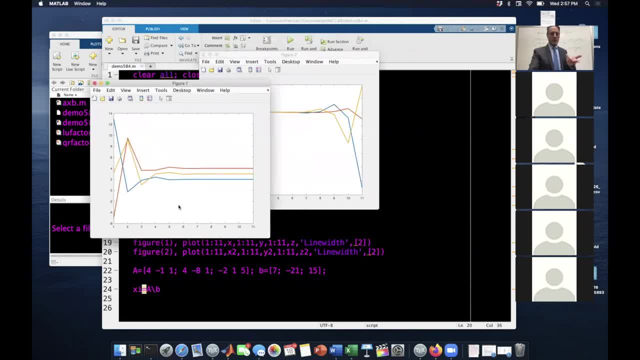 like iterations can converge. Look at this. They do beautifully in the first one. Iterations can do things like diverge, go to a plus or minus infinity. In fact, it seems to be what's happening. It's happening with these guys. 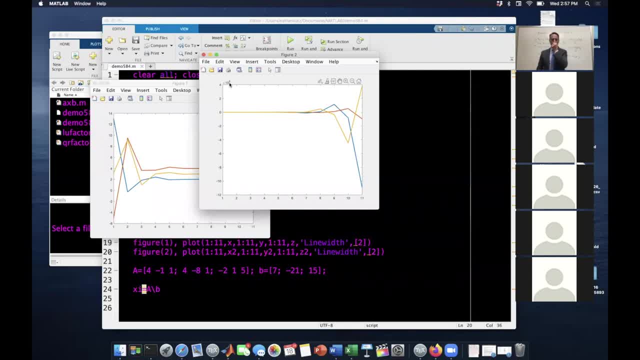 Notice this number up here: 10 to the 5.. So already you started with values that were reasonable, whatever order one values, And now they are five orders of magnitude bigger after only 10 iterations. In fact, they're going to infinity very quickly. 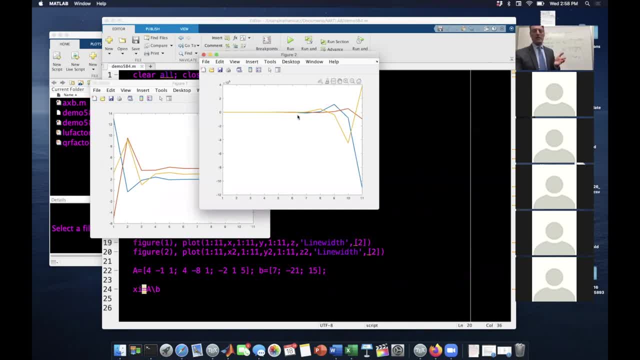 What we know is the answer. this one converged to the answer and this one did not. So the initial hope like say, hey, look at this, Check out this, This magic trick I just did. And the magic trick I did was say 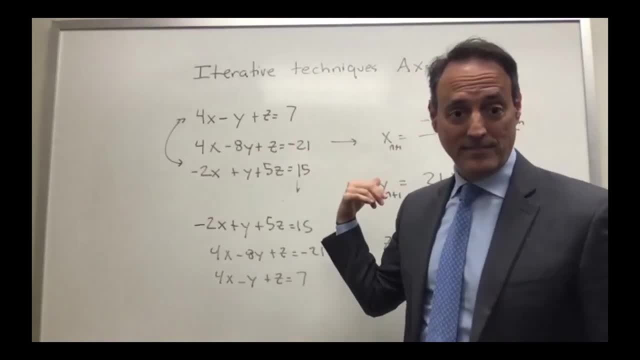 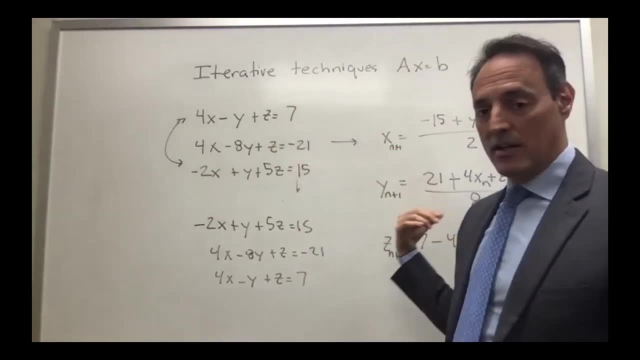 just take the governing equations, rewrite them, iterate, And it works. It got to the solution. I just iterated on that thing. It worked. But then I just did the same equations, did an iteration, and it blew up. So what's going on? 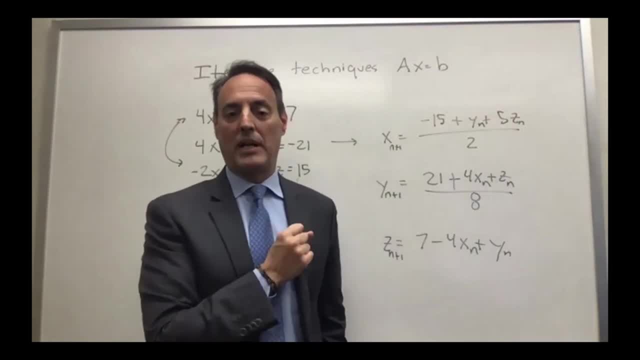 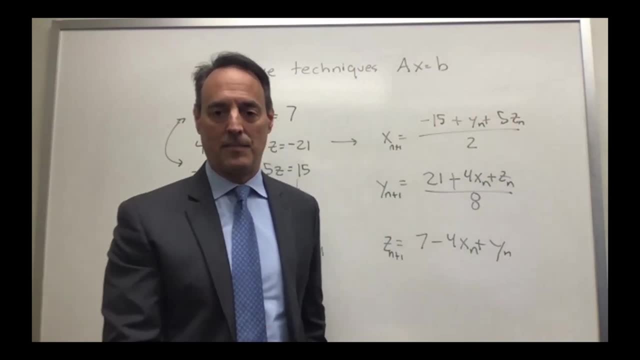 Obviously, you don't want to use a method that is liable to break like this. What you'd like to do when you solve equations is you want them to work consistently. OK, So let's talk about the difference between these two sets of equations. 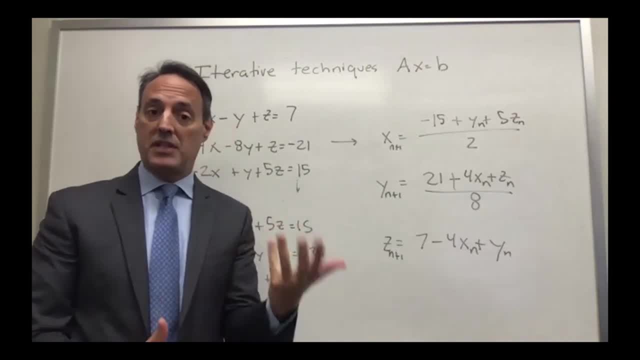 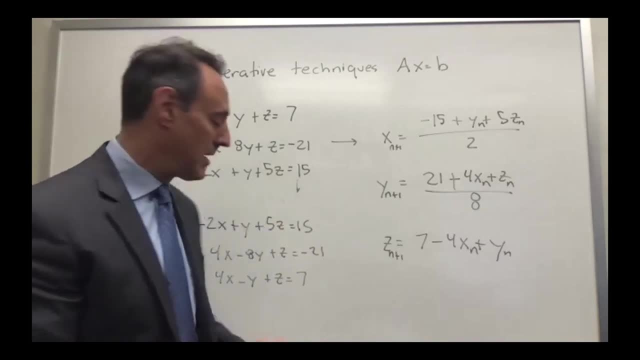 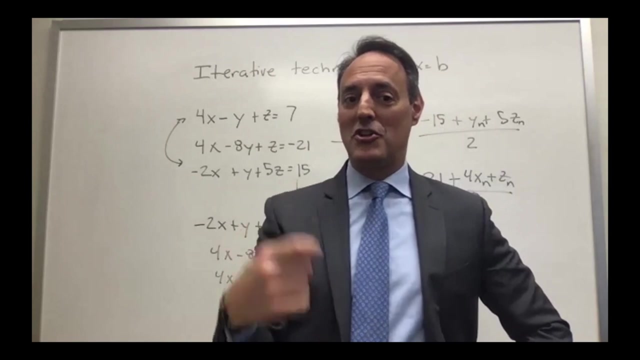 And it's going to highlight a really important part of iterative schemes, which is having to do with the diagonal of a matrix And the diagonal of a matrix. remember when we did power iterations with eigenvalues. remember how the largest eigenvalue would show up. 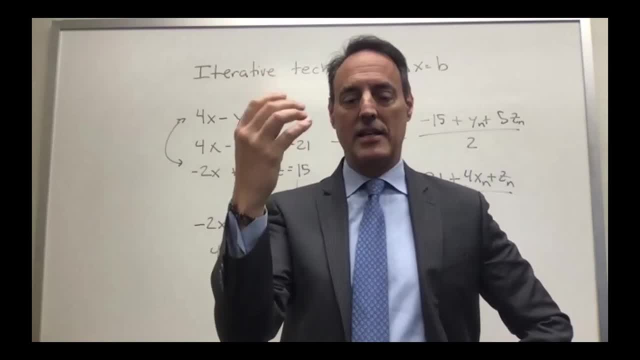 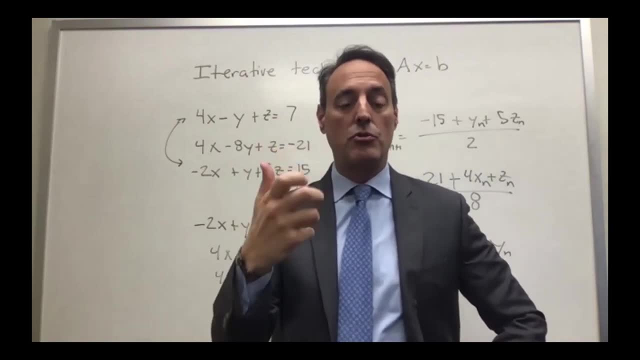 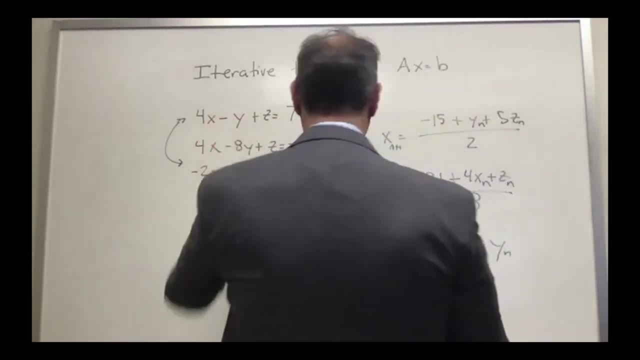 or the eigenvalue closest to my parameter, mu, which would be highlighted, And all the iterations. everything would go away to 0, except for the largest one, which was due to the power iterations. So what we're going to talk about here is: what's the relationship between that and these? 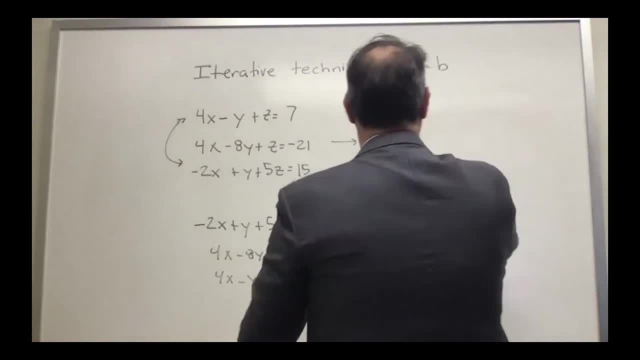 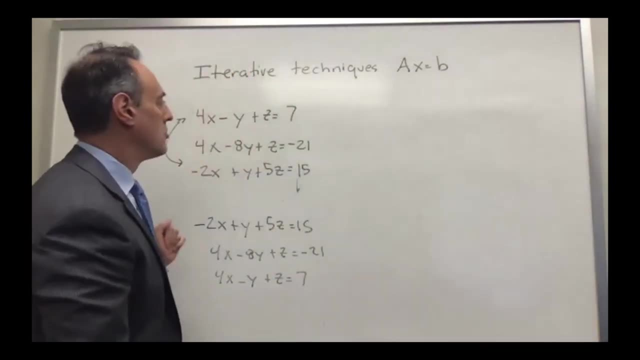 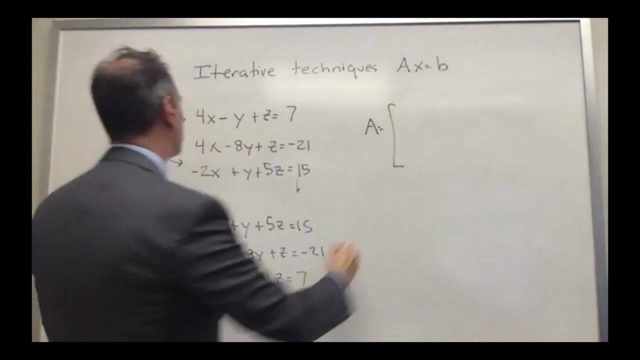 techniques that we've developed here. OK, This has everything to do with the matrix A. in these two cases, We can agree that they're the same governing equations, same solution. But the way I've written this one, let me write it with the matrix A. The matrix A in this case. 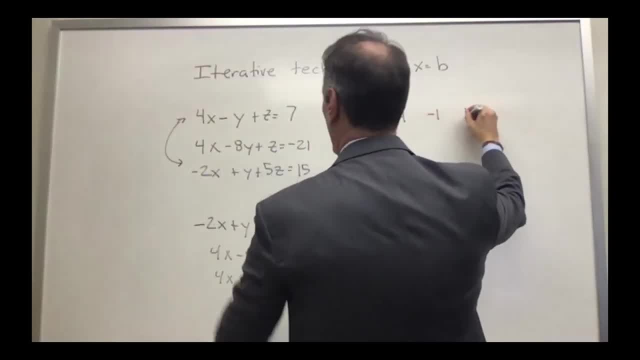 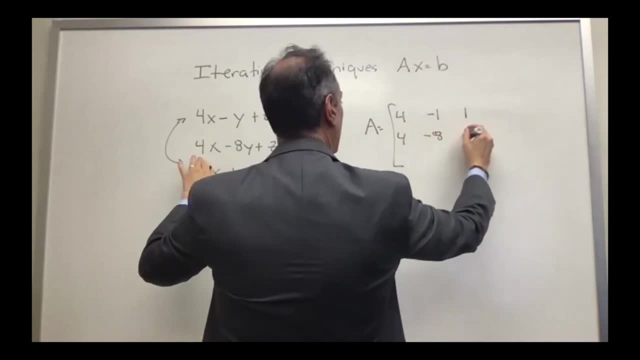 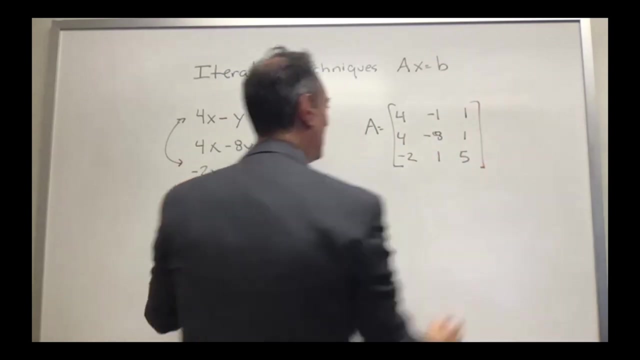 is 4, negative: 1, 1. from here The matrix here is 4, negative 8, 1.. And then here it's negative: 2, 1, 5.. And then the B is this here, But I'm just going to focus on the matrix. 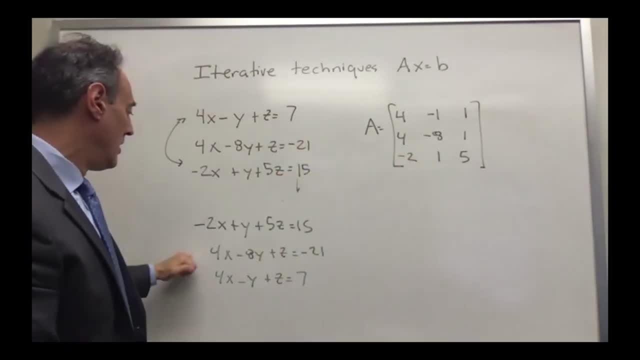 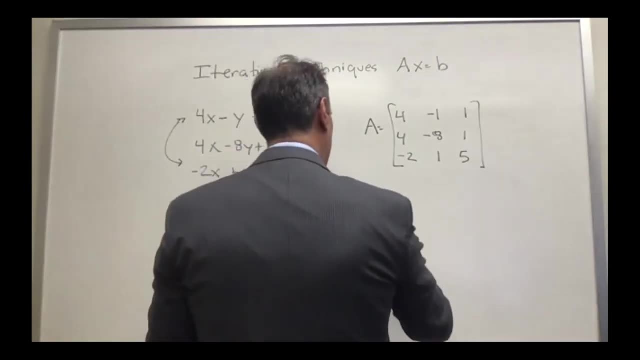 I'm just going to focus on the matrix A. When I look at this matrix, which is the same solution, all I've done is interchange rows, columns. All I'm going to do is switch this with this first and third rows. 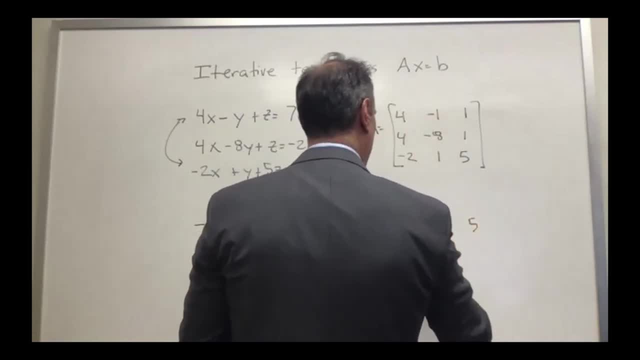 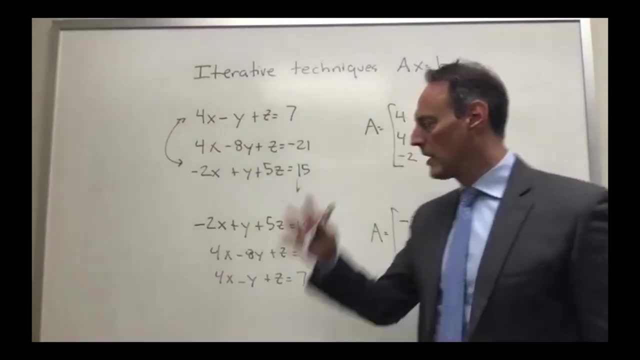 So I'm going to get minus 2, 1,, 5,, 4, negative 8, 1,, and then 4, negative, 1, 1.. OK, Same solution, But here's the big difference. I want to highlight it in here, which. 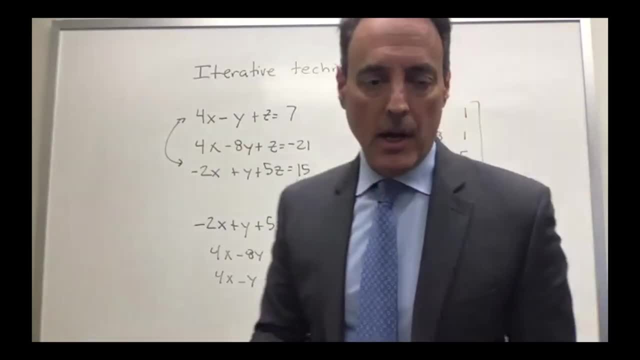 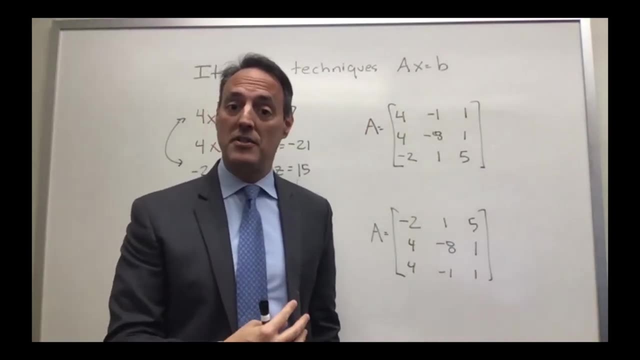 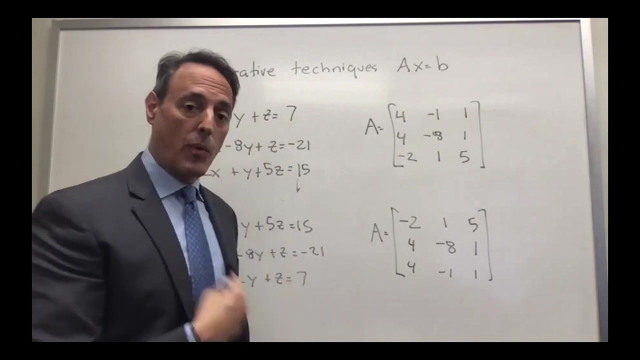 is when you have governing equations like this, and we're going to talk more about how these iteration schemes work, but the difference between these two formulations is what's called diagonal dominance. OK, And in particular, the way you define whether a matrix is diagonally dominant. is you look at? 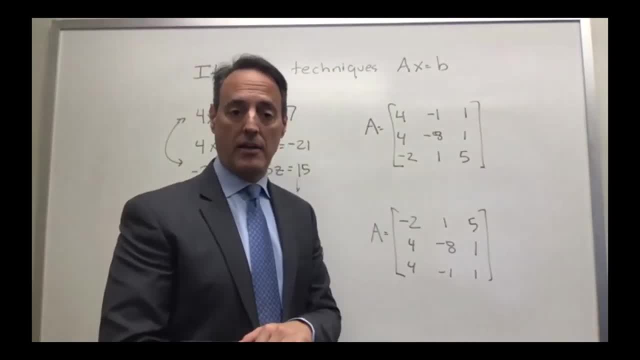 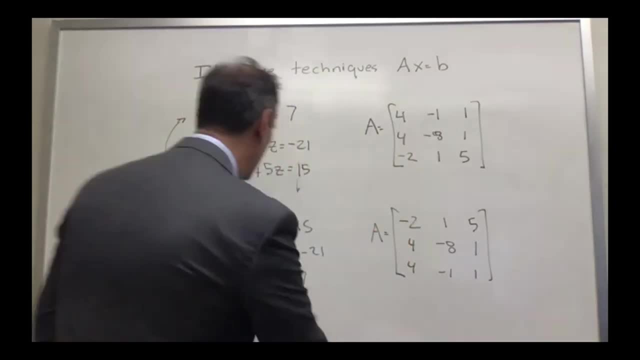 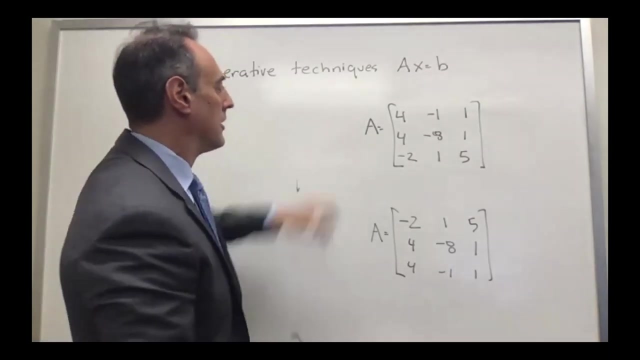 for each row. it's the absolute, Absolute value of the diagonal And you see, is it bigger than the sum of the rest of the terms. So what do I mean by that? I'm going to erase this And let's look at what diagonal dominance means here. 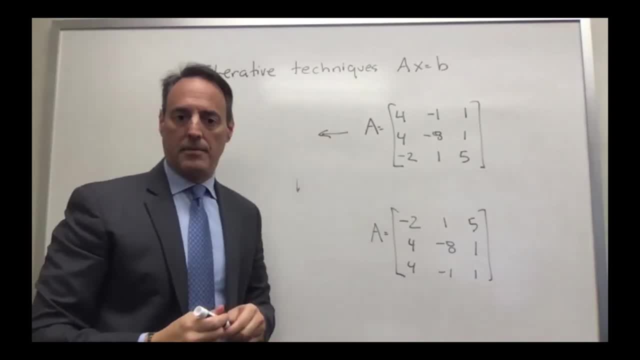 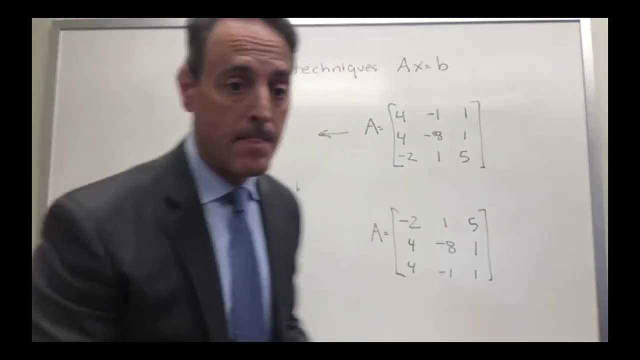 Is this matrix diagonally dominant Or what's called stricter diagonal? About the diagonal, What's that? Some of the diagonal, the same as the triangle, The trace of the matrix, The sum of the diagonals? yes, OK, thank you. 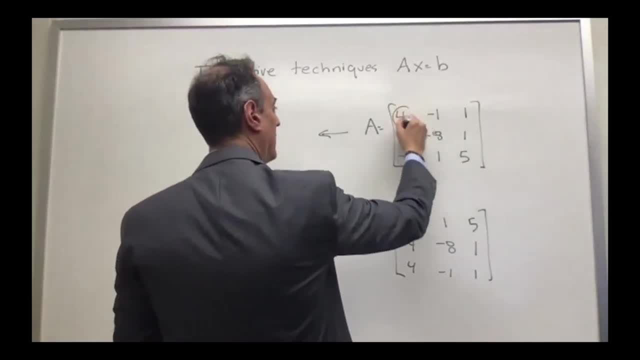 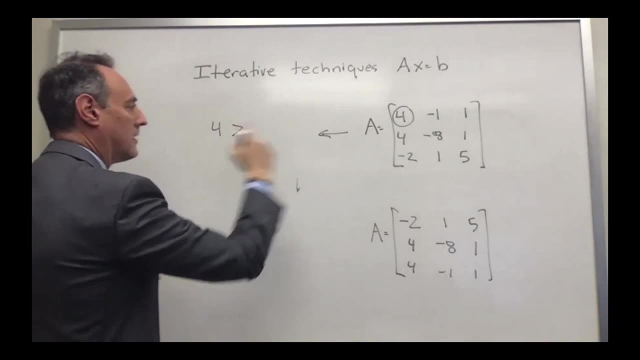 Yeah. So what I want to look at is the diagonal term here is 4.. Is 4, the absolute value of 4,, which is 4,, bigger than the sum of the absolute value of the other terms, which is 2?? 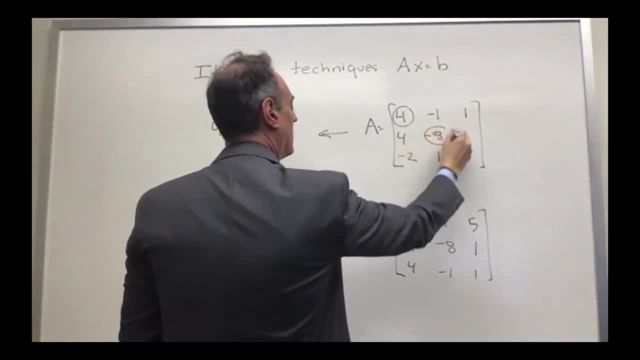 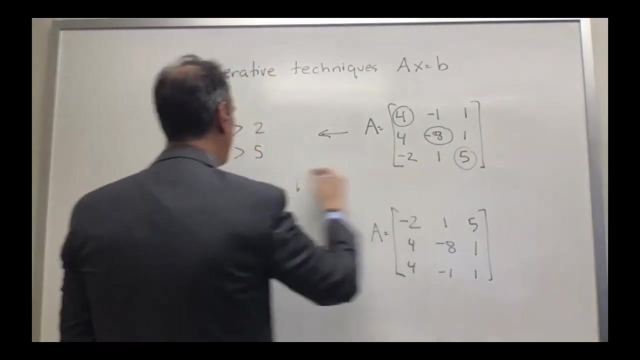 It is here's. the diagonal is 8, bigger than some of the other terms. the rest of the row Bigger than 5, it is. Is 5 bigger than the sum of the other 2?? Absolute value of the 2?. 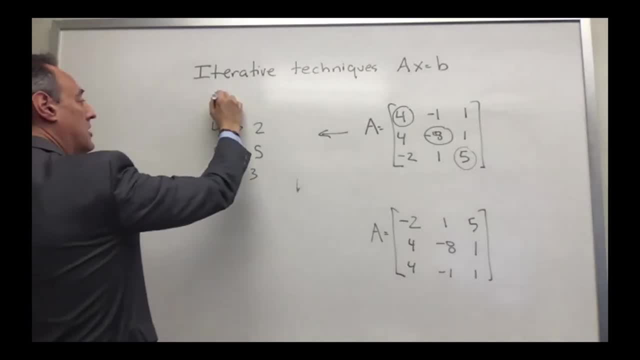 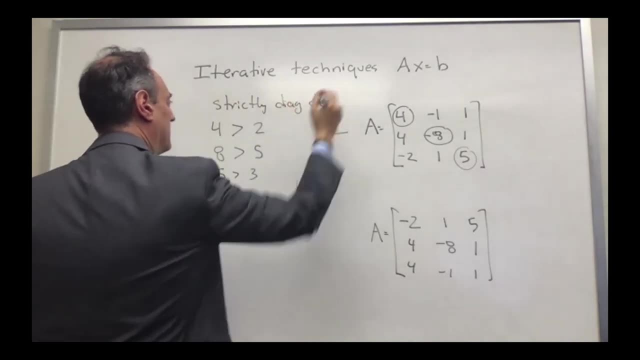 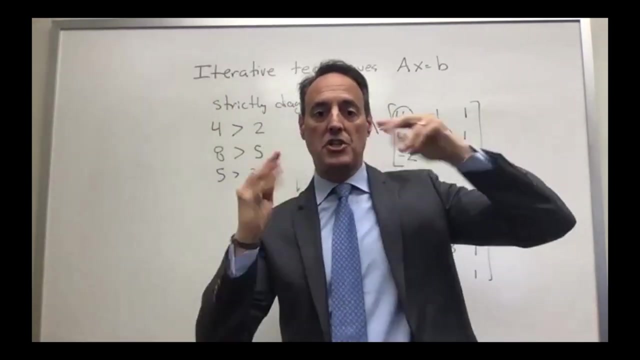 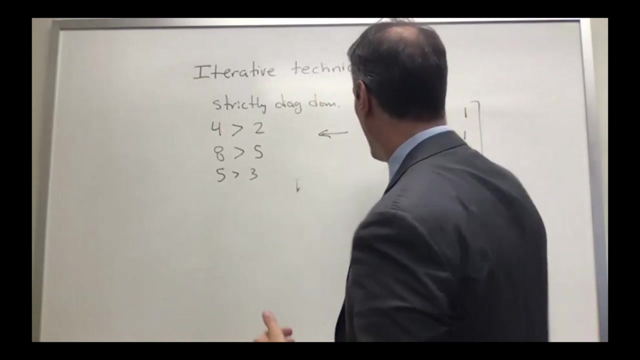 5 is bigger than 3.. So this means it's strictly diagonal dominant. This diagonal dominant is really important because it's very much like when we iterate on eigenvalues. It just As you do The power iterations. essentially everything disappears except for the diagonal term. 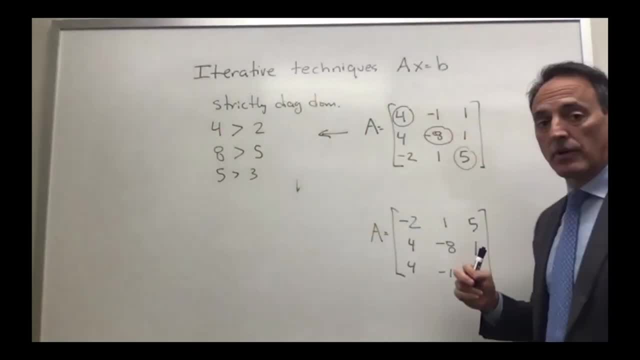 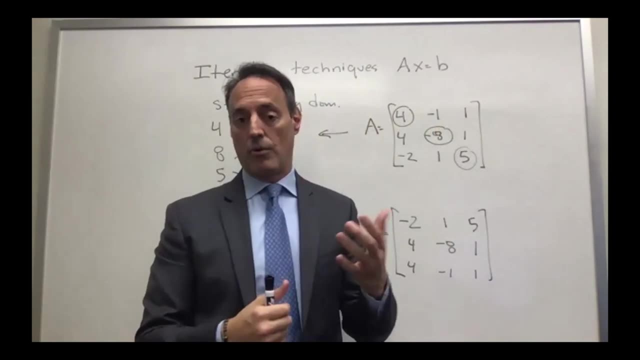 where this is what is converging along these directions. OK, like I said, we're going to spend more time talking about more sophisticated methods for this And, in fact, the method we used- we're going to come back to in a minute- was just. 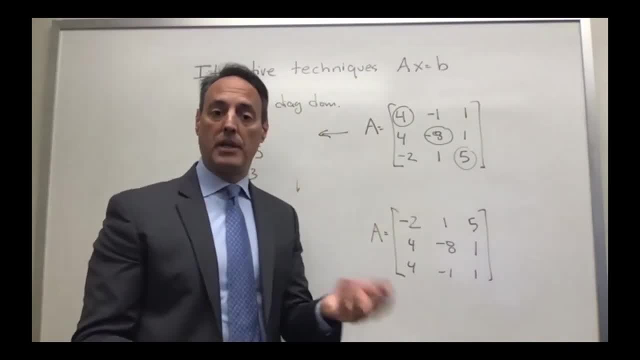 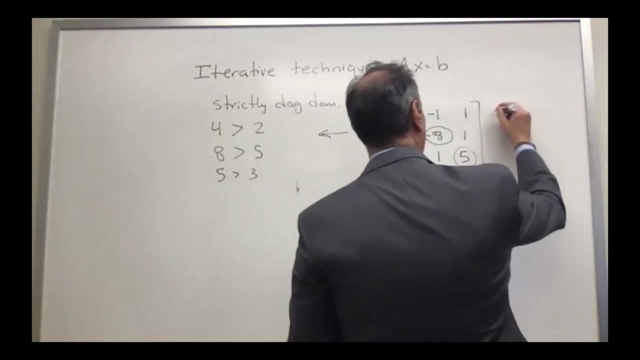 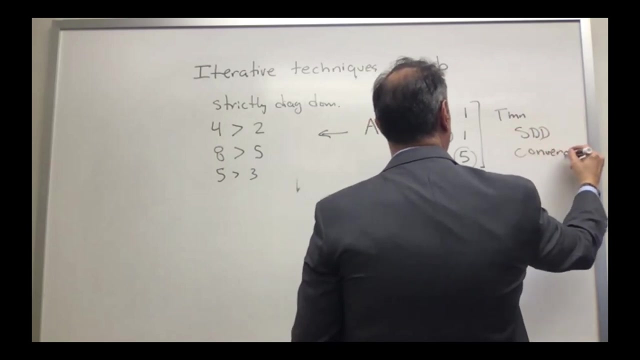 if we take the current value and update it, it's called a Jacobi iteration. OK, so Jacobi iterations if it's strictly diagonal dominant. there is a theorem which states that if you are strictly diagonal dominant, you converge Guaranteed. 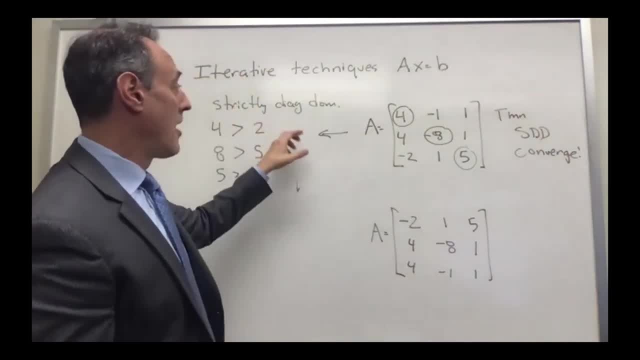 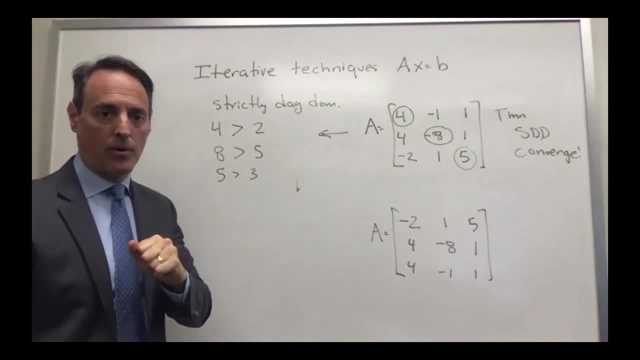 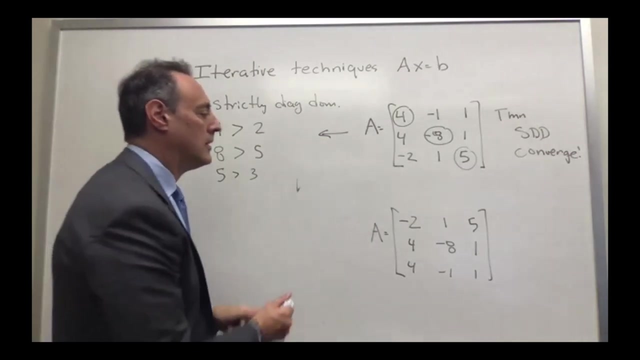 Great And strictly diagonal. dominant means you are greater, not greater or equal to greater than OK. that's an important point to make. Let's talk about this one here. What about this matrix? Same solution, right? I mean we all agree. 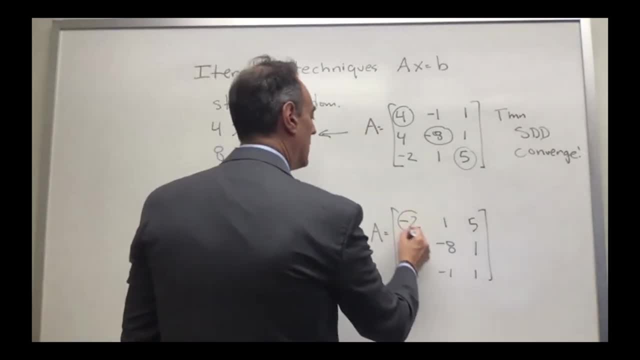 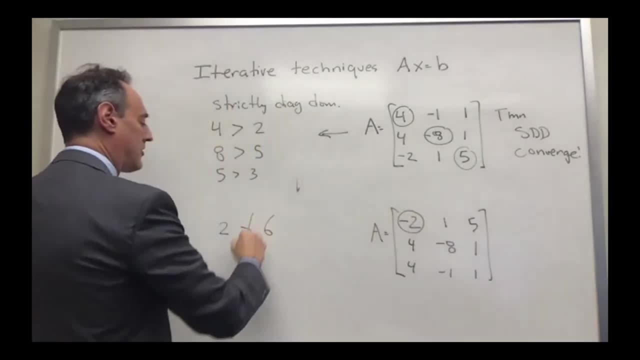 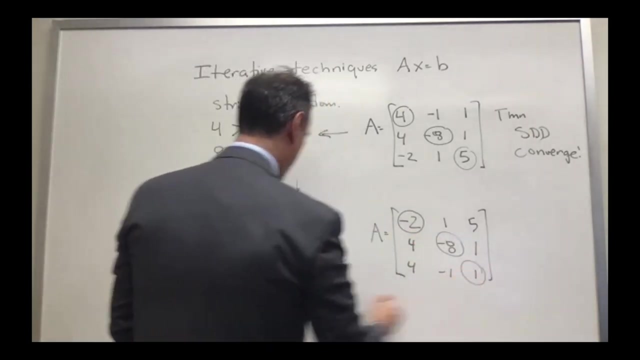 All I did was interchanged rows. I go grab the diagonal. term Is two bigger than some of the other two, six, And it certainly is not. The second row is eight bigger than some of the other two columns: Five it is. Finally, this diagonal was one. 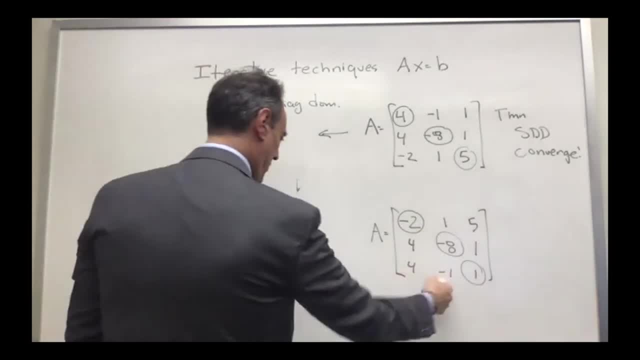 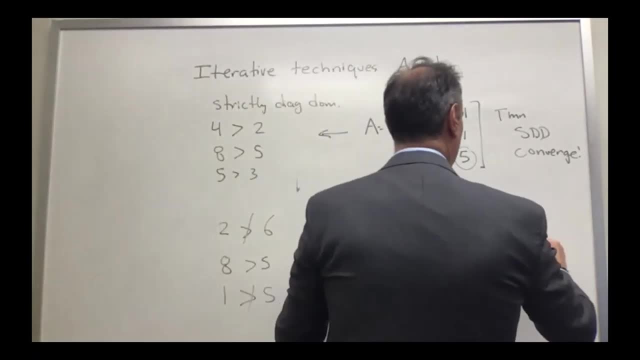 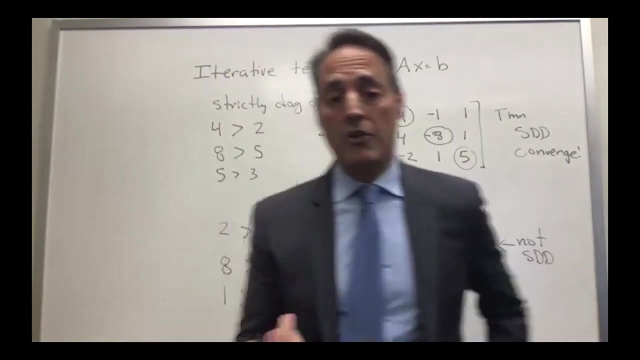 OK, It's one. Is that bigger than some of the other two? opposite value of two. Five. it's not. So this is not strictly diagonal dominant. So what's interesting about it? if you're not strictly diagonal dominant, you can't say it's going to diverge. 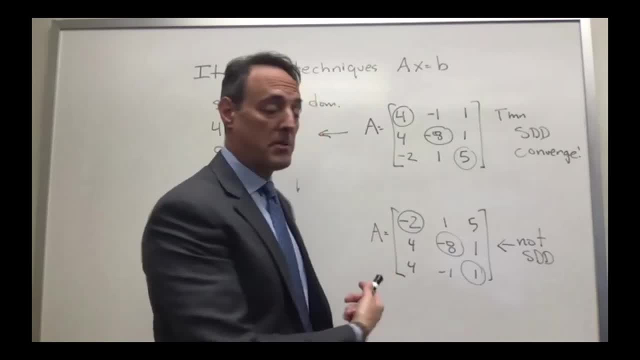 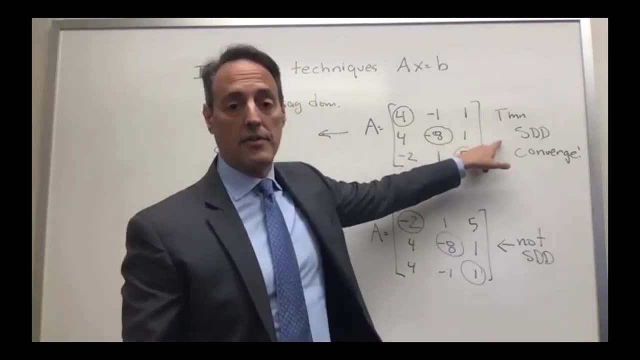 You can't say anything. You can't say it's going to convert. Sometimes it doesn't have to be strictly, It's not strictly diagonal dominant, It still converges. OK, this is only a guarantee. It's a guarantee of convergence. 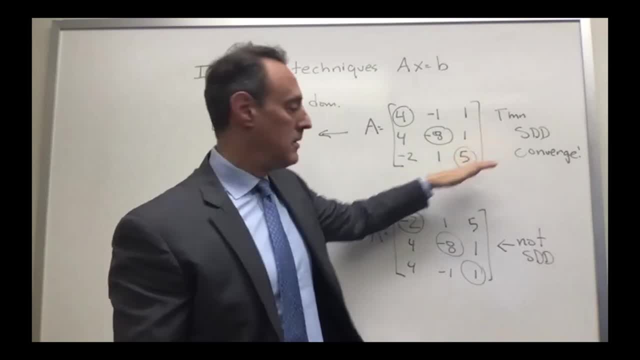 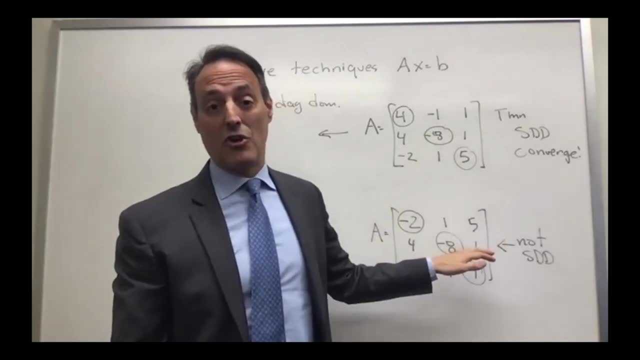 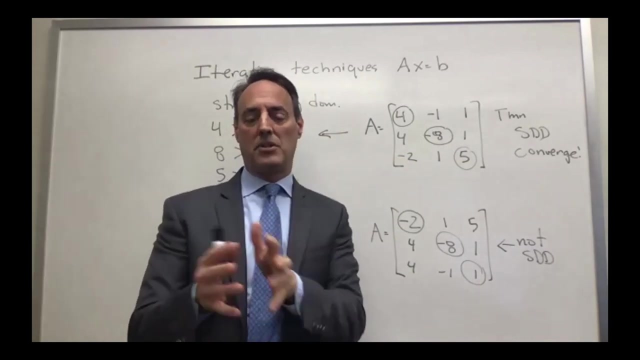 If you don't satisfy strict diagonal dominance you can't say anything about it. But generically, if you don't satisfy strict diagonal dominance, it just also means your solution might blow up, which is problematic, Right? Because if you're trying to guarantee that, I put this in. 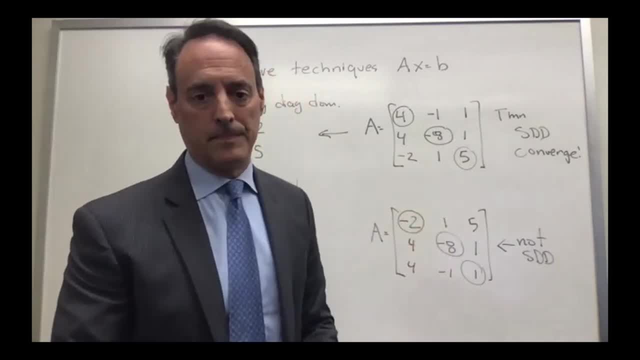 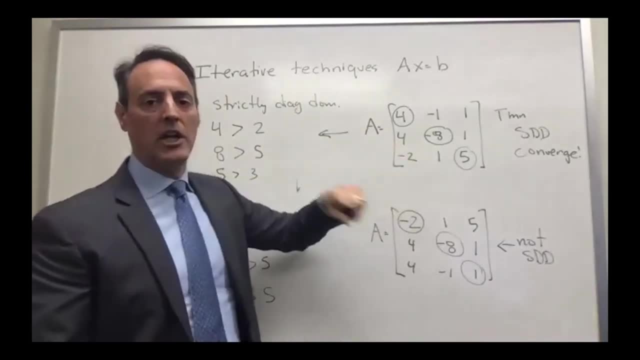 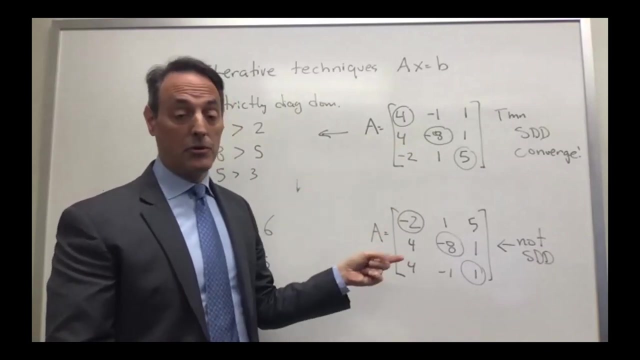 and get a solution. this is going to be a problem for you, OK. So strict diagonal dominance matters, And if you have it, If you iterate, you converge to the solution. If you don't have it, you could blow up. 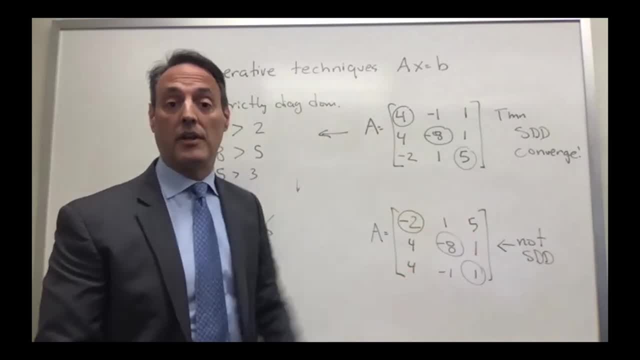 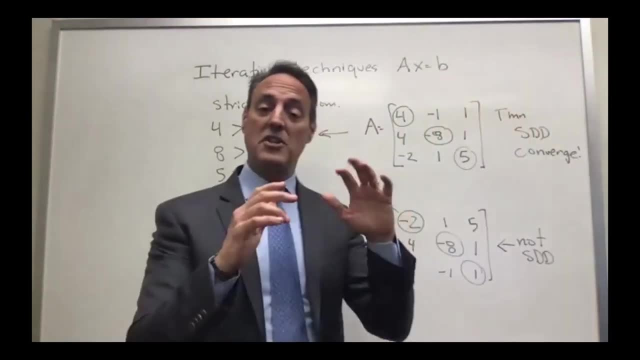 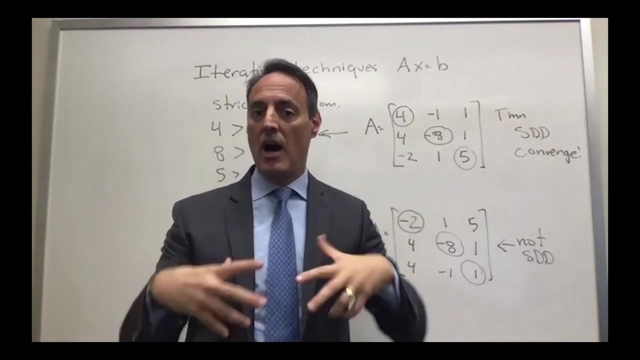 You could converge You just you don't know, You can't say anything specific about it. OK, so this is going to be of. this is an important observation for what comes next in the next two lectures, which is we're going to build on these themes of iteration techniques. 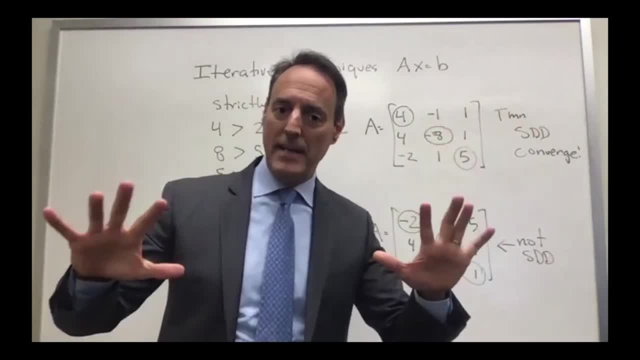 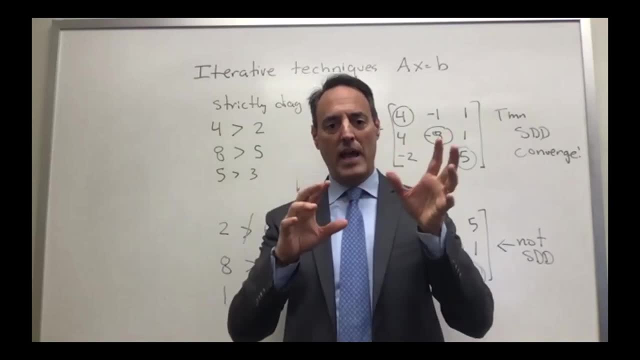 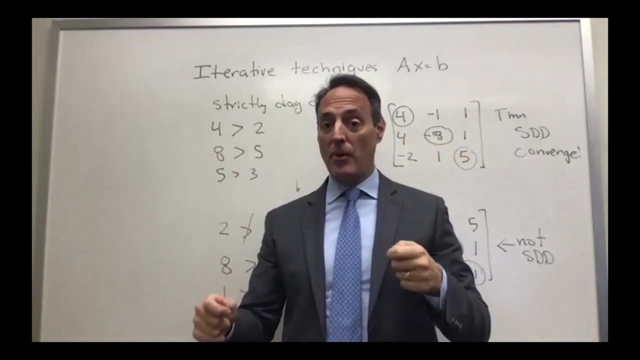 for solving x equal to b And notice how fun The mentally different this is than what we've been doing. Everything we've been doing in x equal to b is having a progressive way to just get to the solution. We can even say it within order and cubed operations. 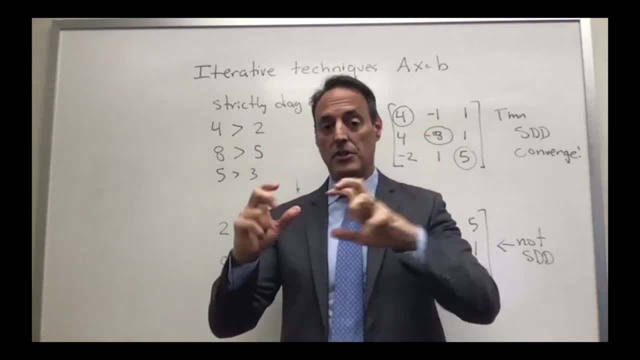 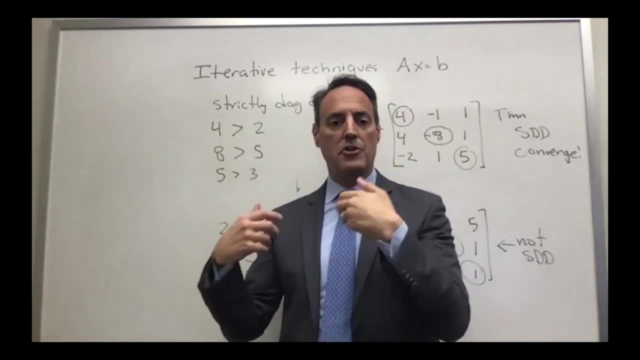 I am guaranteed to get to the solution because there is a series of operations. As long as that matrix isn't singular, I just perform these series of operations. OK, they're deterministic. I get an answer here, Here, Here, Here. 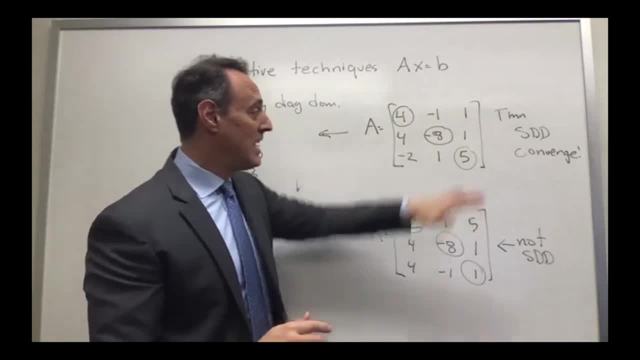 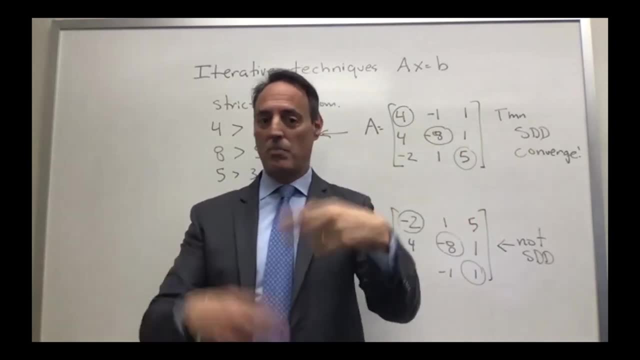 I start with a guess And, by the way, this convergence guaranteed for any guess. We'll do it in a minute. We'll just play around with some guesses. Doesn't matter what you guess If you have a really bad guess it. 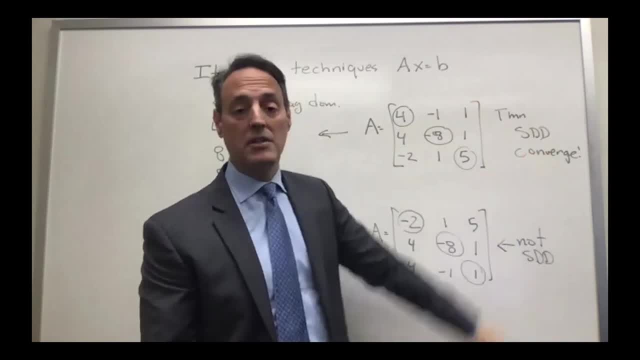 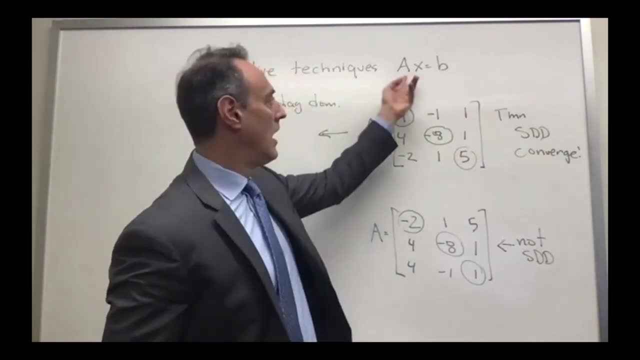 might take more iterations to get to the solution, but guaranteed to converge Right for any guess and a lot of these algorithms. what they guess is just say: oh, I'm going to solve x equal to b. I put it in this form: 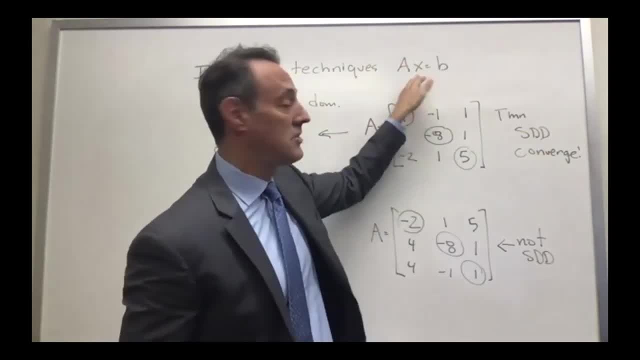 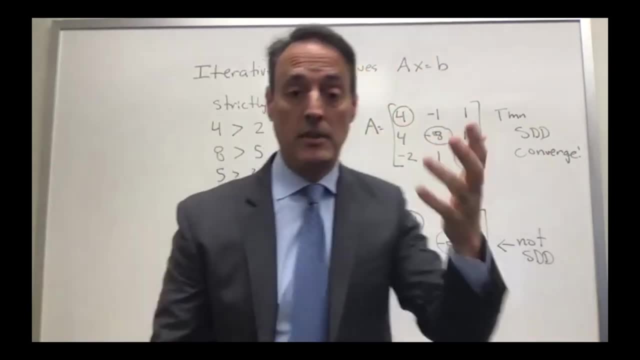 I don't know. Since I don't have anything else better to guess, I'll just guess that x is 0. So you start there and it iterates to the solution. OK, let's show it. I'm going to show it on this method. 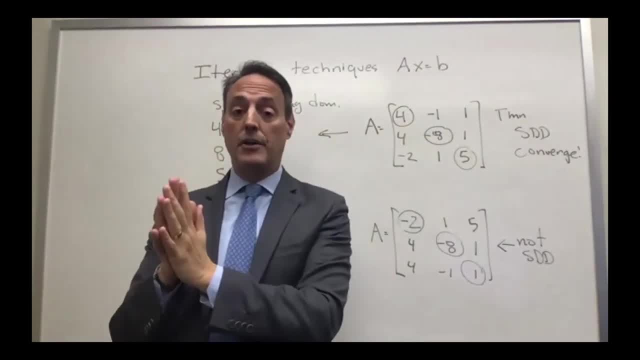 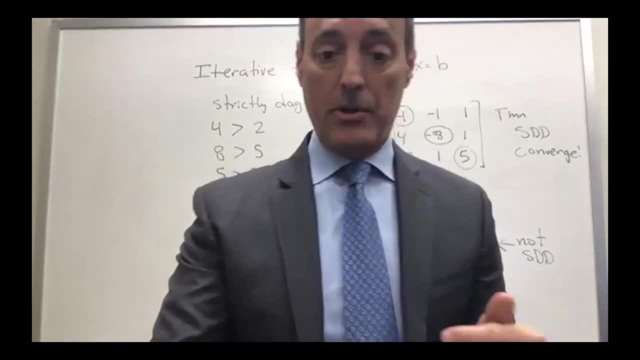 In fact, the iterations we did here, which is, you take your current values To update them all. it's called Jacobi iteration And let's talk, Let's show you what happens when we change guesses. All right, so I'm going to share screen. 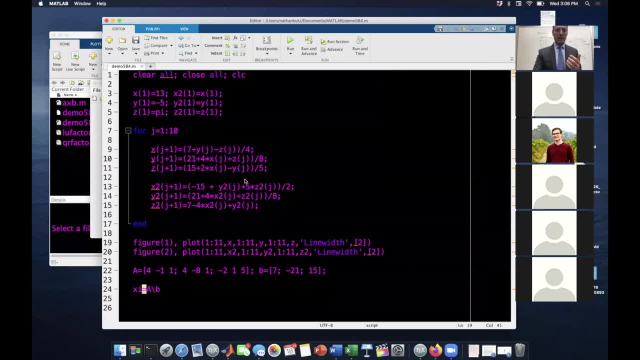 Sure Boom. All right, So we'll come back to here And remember- I just picked these randomly- 13, negative 5 pi. I could also just pick here, which is like, if you don't have any better to pick, you can 0,, 0, 0 is. 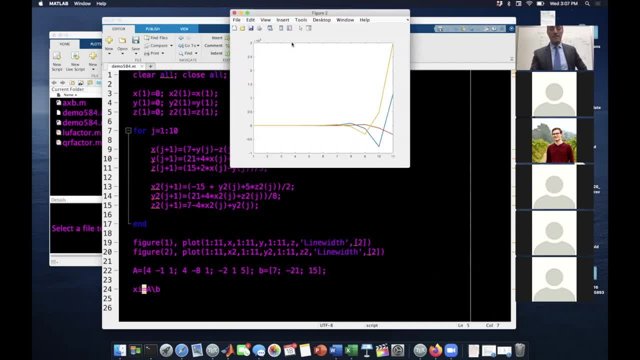 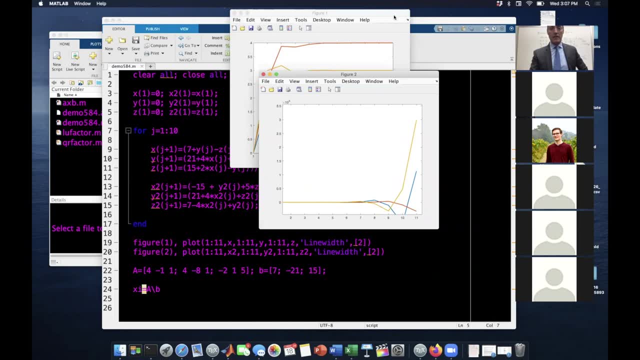 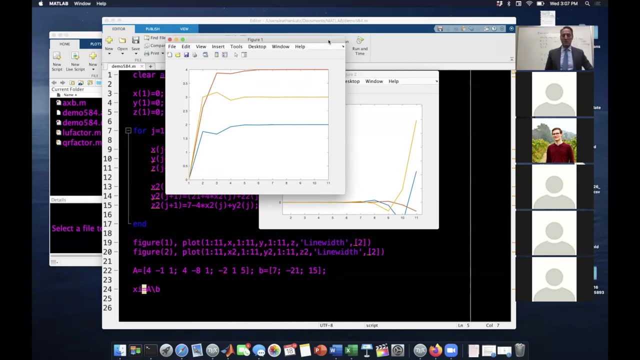 perfectly as good as any other guess. You run that Again this is the one that blows up here, And then here's the convergence to the solution. So again, I just showed you: OK, Different guess still converges really quickly to those solutions which are 4,, 3, and 2.. 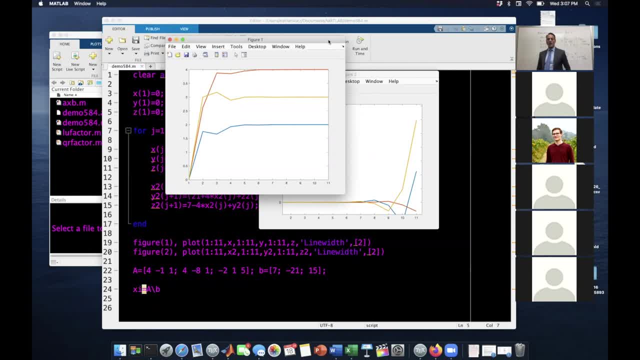 OK, I'm going to show you one other thing we can do with this And notice. so, first of all, I want you to know something here: By around six or seven guesses it's converging, right? This one here, of course, just blows up. 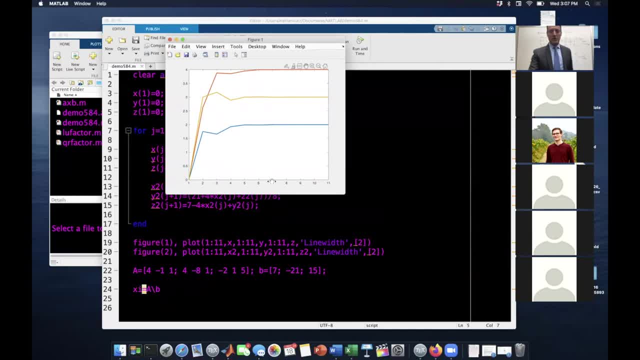 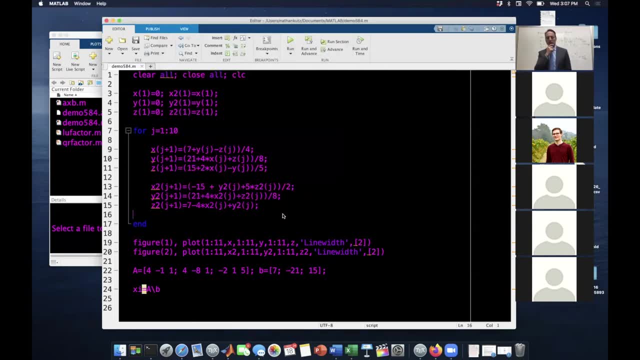 So let's just ignore it. So about six or seven iterations And it converges Pretty close. I want to do one other thing here. I want you to start to look at this algorithm. Notice something. When here's this algorithm, I start out. 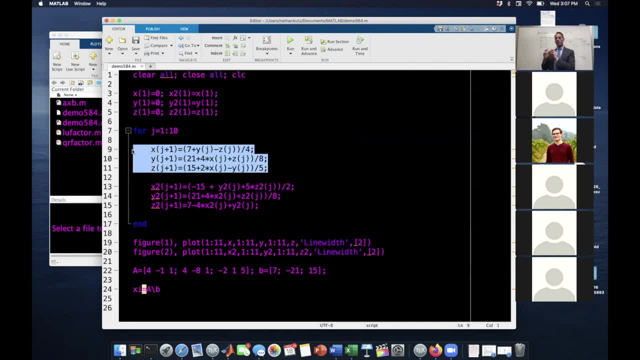 with the initial guess of x, y, z, And then I use those values to get me new values of x, y, z. Now, presumably, when I update these values, I'll stop sharing for a minute. So the idea is: I give you a guess. 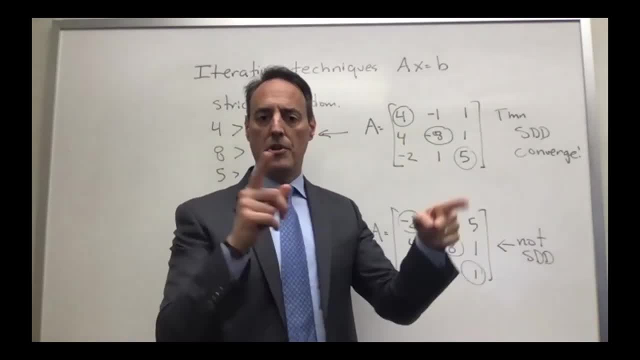 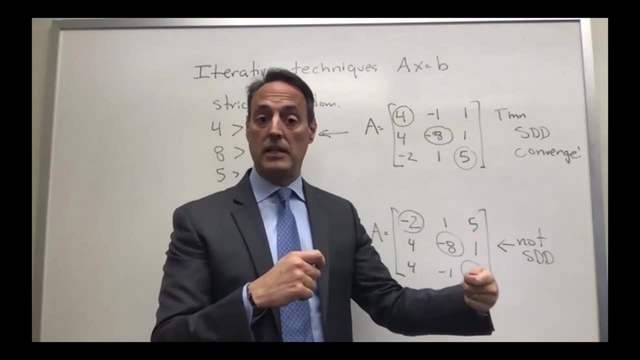 I use that guess to give me new values, New values of x, y, z. But notice, in this algorithm I first say let me update x, Then let me update y, Then update z. That's called Jacobi iteration. 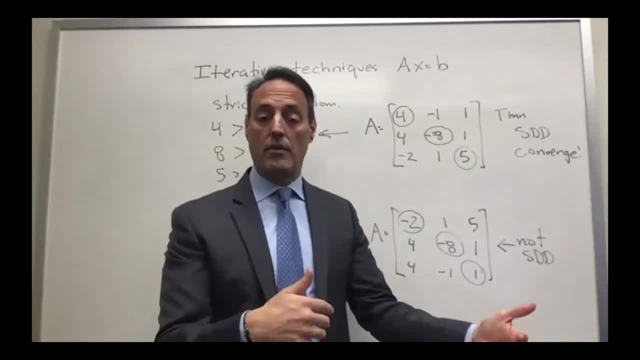 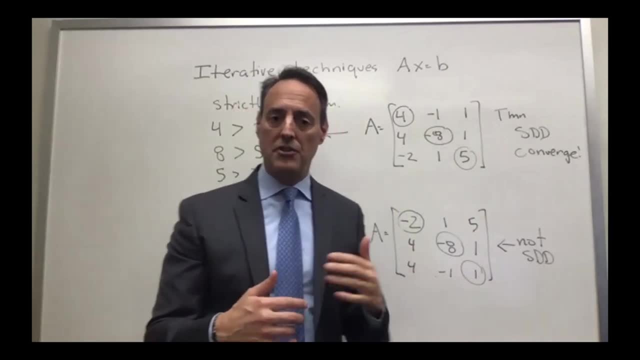 I just take the previous values and I create updates for all of the values. There is a way to improve this. what's called Gauss-Seidel And what Gauss-Seidel says. well, wait a minute. In the first step, you updated x. 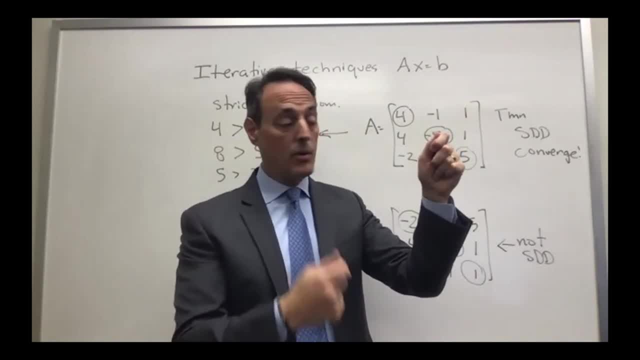 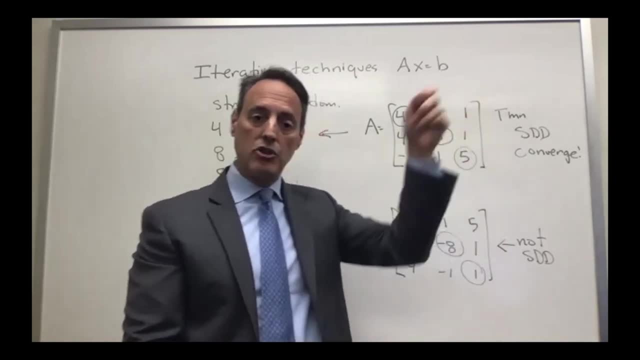 Why wait till the next round of x? Why wait till the next round of iterations to use that x? In other words, if I already have this new value of x, I can use it immediately. I don't have to update all the values. 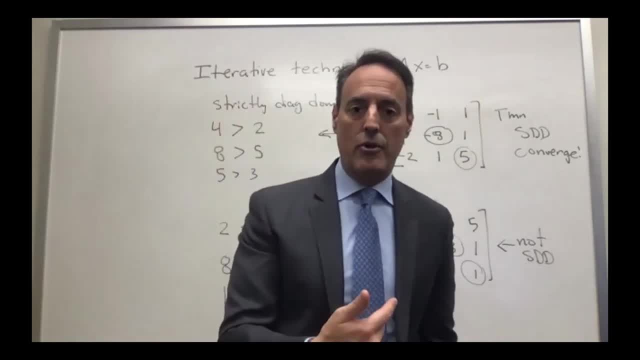 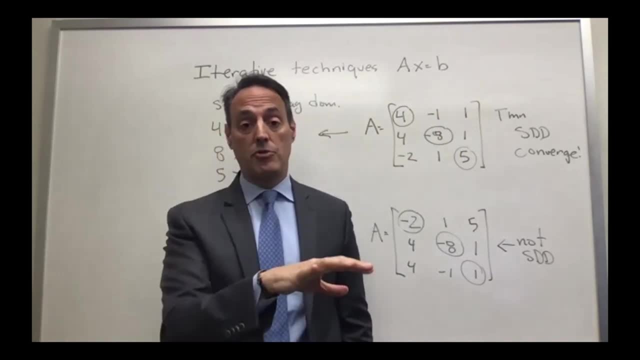 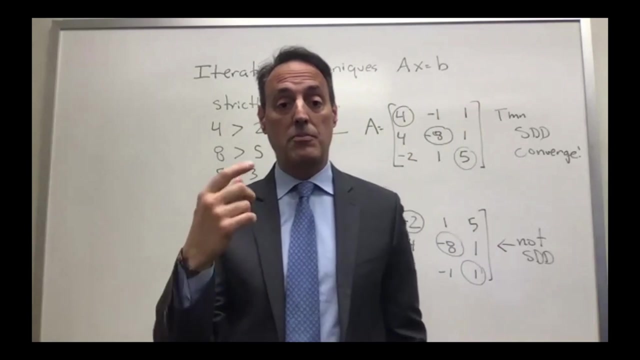 I can use that value as soon as I get it in my current set of iterations. So what I'm going to do is show you an update to the code which takes from Jacobi iterations to Gauss-Seidel iterations, which improves your performance. 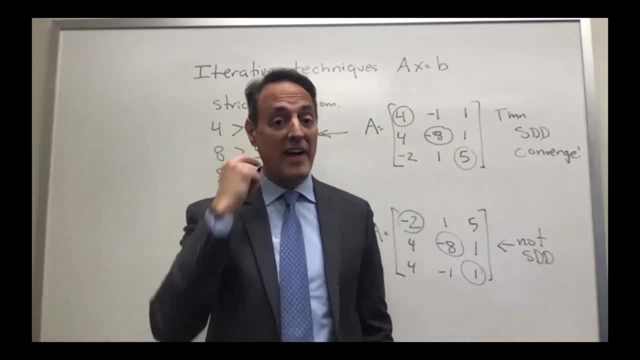 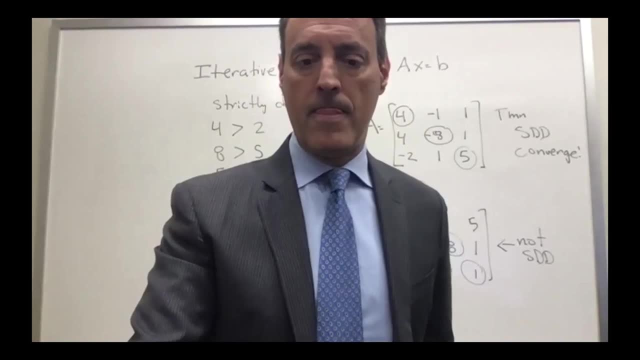 Because presumably, every time you iterate, you get closer, And so I'm just using a better value faster. So let me just show you where this would change in the code. So here we are. Here's the code. So what I'm talking about specifically is look. 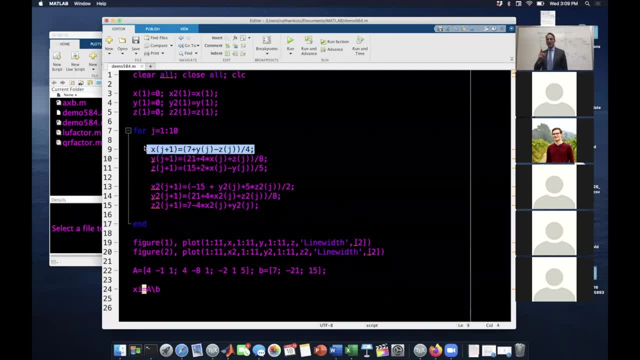 right here in this first line. I just improved my value of x. presumably. I grabbed the y's and the z's and I got a new value: x of j plus 1.. x of j plus 1 should be better than x of j. 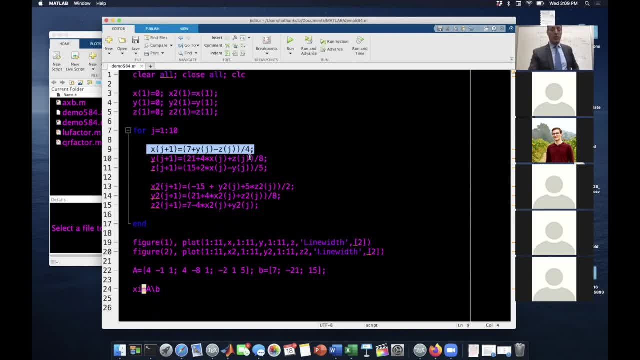 My second line of the code y's of j plus 1 is equal. to look at it, there's an x of j in there. But why would I use my old value of x of j when I have a new value of x of j plus 1?? 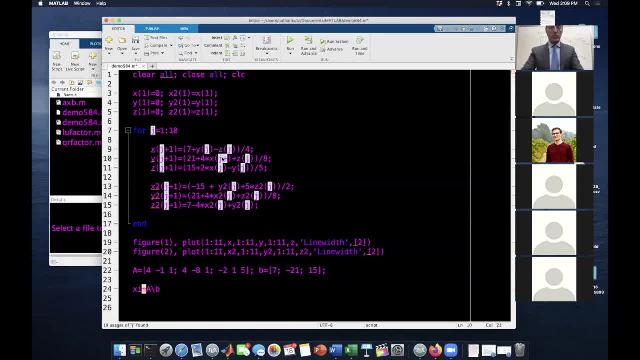 So in fact, right here I can immediately use x of j plus 1.. So I'm using my update as soon as I get it. So I take the x of j. I already have x of j plus 1. So use it immediately. 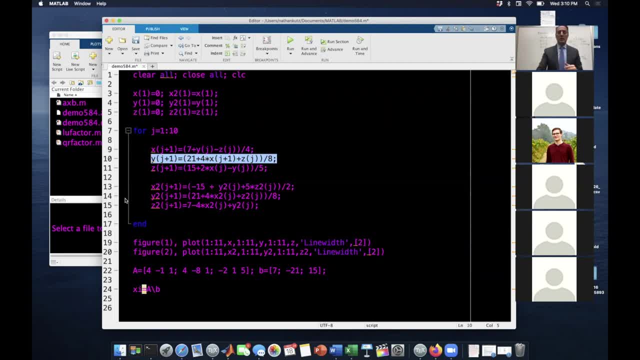 Specifically on that next line. And then I say y of z's of j plus 1.. Notice, it requires x of j and y's of j, But I just have improved values of both of these So I can put in here plus 1, plus 1.. 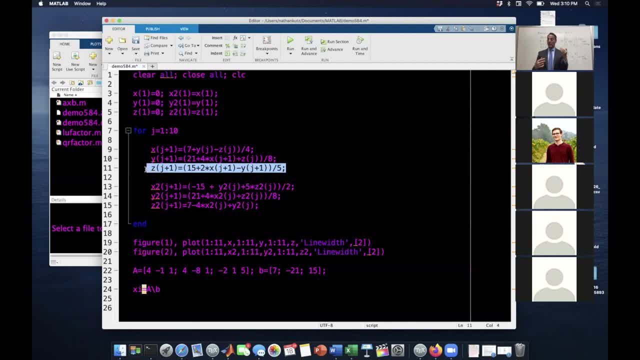 And now the idea is that I should get a better value of z, of j plus 1, because I've already used better values of x and y. Was there a question, By the way? Come on, No, OK, So this is called Gauss-Seidel iterations. 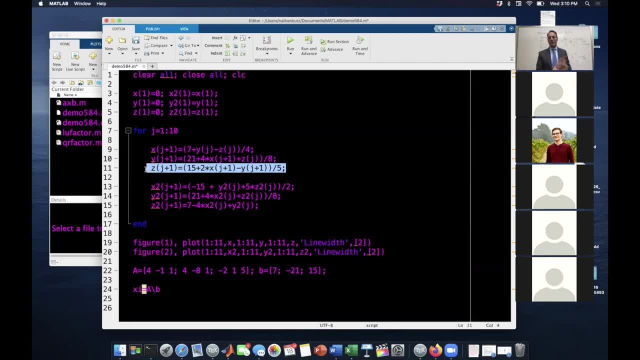 Remember, when we do this coding, it's not just about getting the right answer, It's about how fast can you get that answer and how accurately. So in this case, Gauss-Seidel, you trade this out, not because, hey look, I got a better answer than Jacobi. 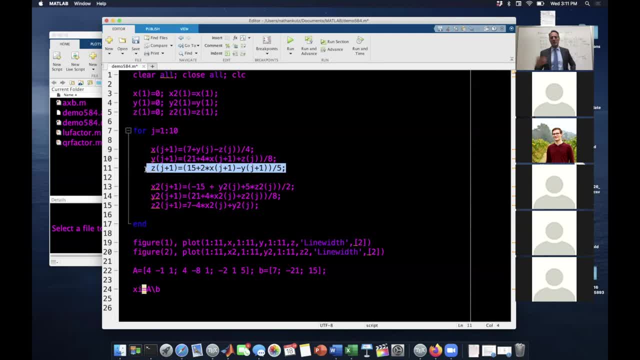 You get the same answer, just that you might be able to get it faster. Remember, computations is all about this combination of accuracy and speed, And so this is getting at the issue of speed. How can I use my results on the fly to get this faster? 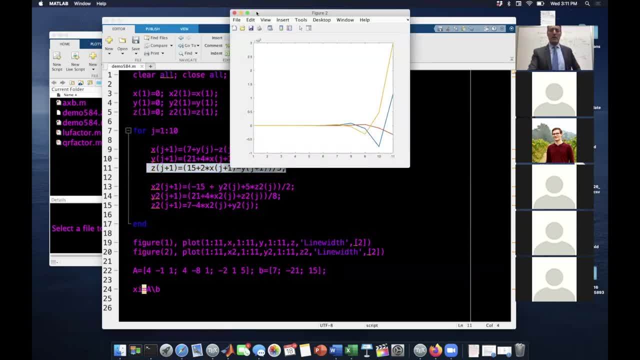 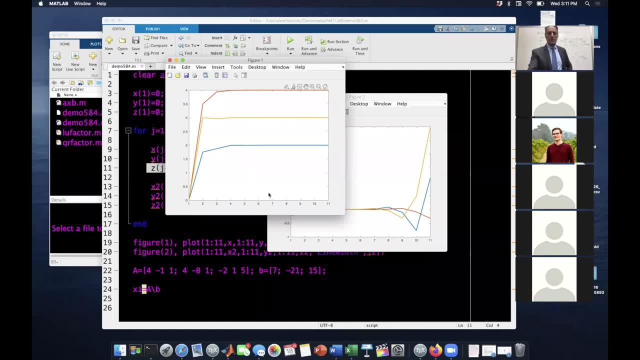 So let's go ahead and run this And let's go dump this out. And I want to show you this. If you remember, in the last plot I showed you it took them to about iteration 6 or 7 to get this to converge. 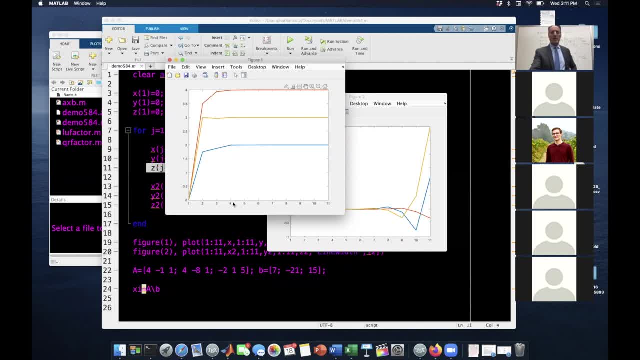 But this thing here is already starting to converge towards that And I want the iteration 4, so three or four iterations- In fact a lot of times if you just look at this quantitatively- I've done this before- where you can just take this simple system. 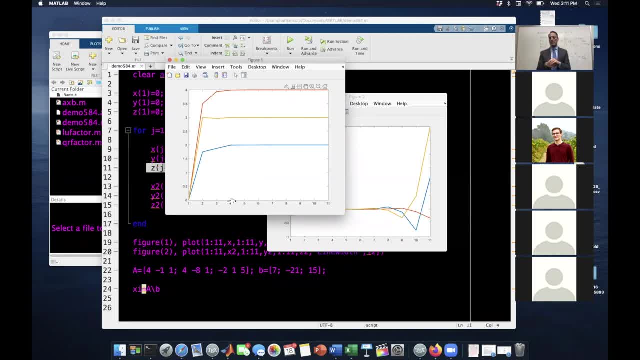 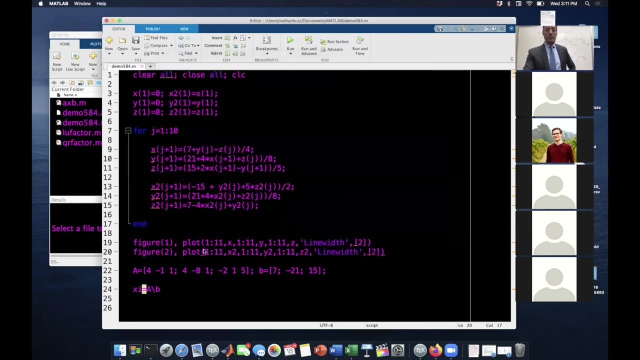 and just say: at what point do they reach about the same error? And usually this Gauss-Seidel often goes about twice as fast as Jacobi iterations. So this is the idea is that you just say: hey look, use your knowledge on the fly as your ability. 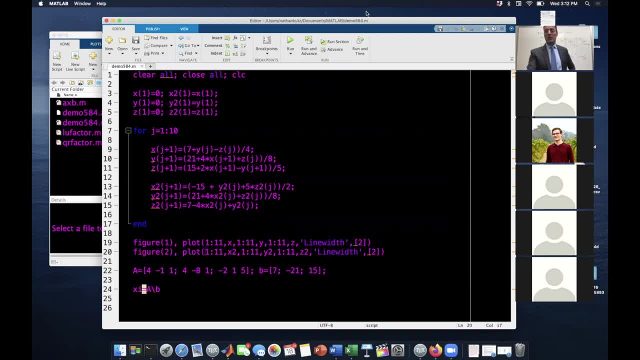 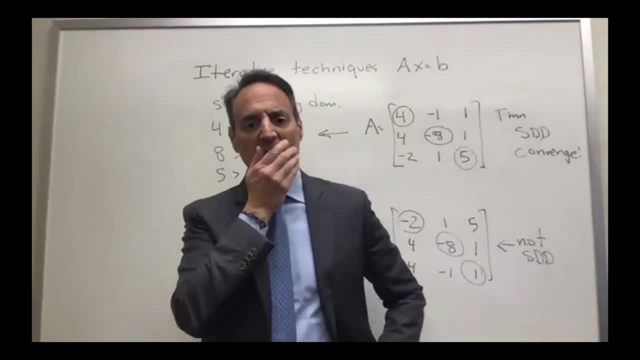 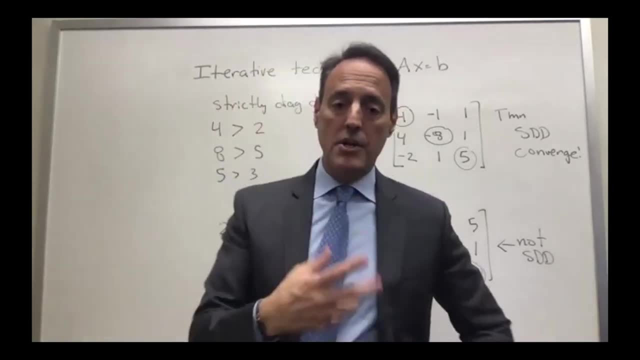 We're building these models And then that's going to converge faster to the solution, And I just showed you that on this very simple example. So this is kind of interesting setting up these architectures, And I want to just highlight one key aspect of where this stuff 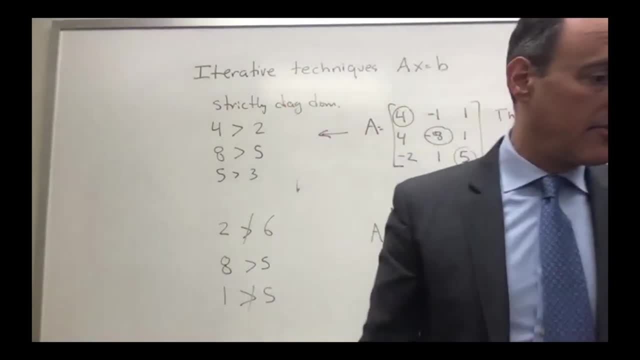 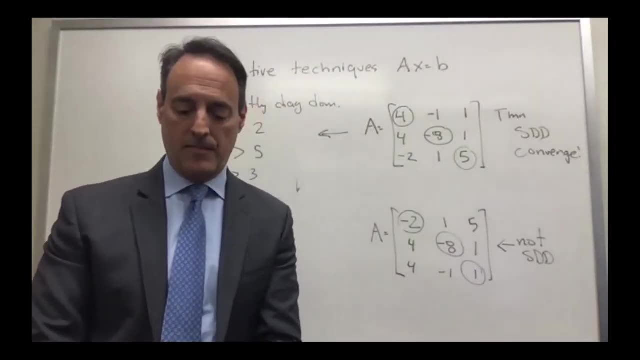 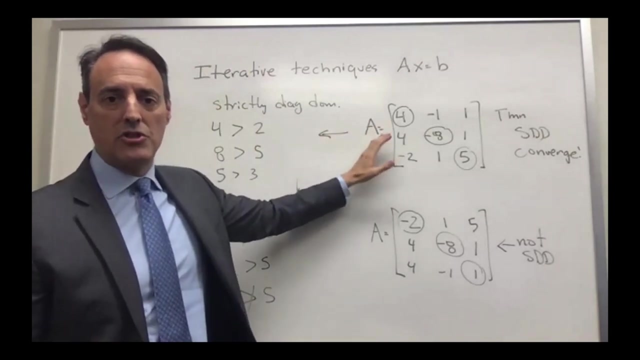 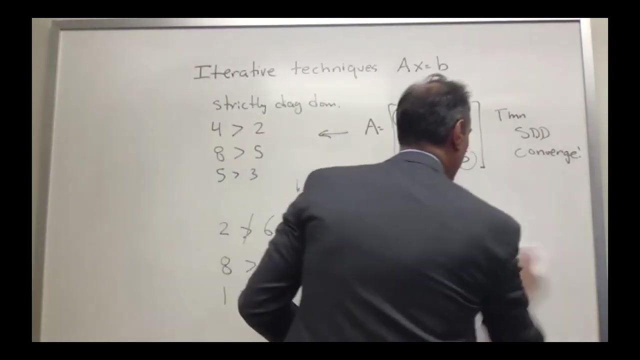 is actually used in practice. A lot of scientific computing revolves around solving high-dimensional, big-scale problems, And a lot of those high-dimensional systems, the matrices that you're generating actually turn out to be matrices generated from differentiation matrices. So, for instance, let me just draw you something: 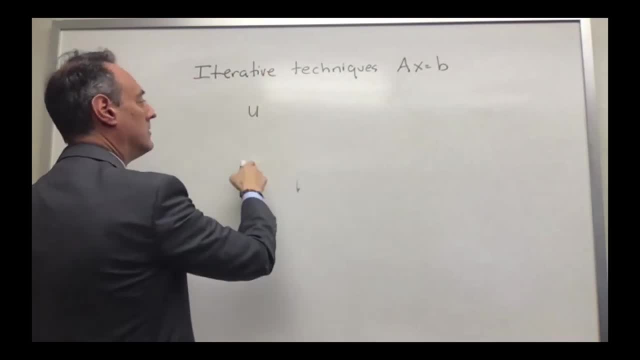 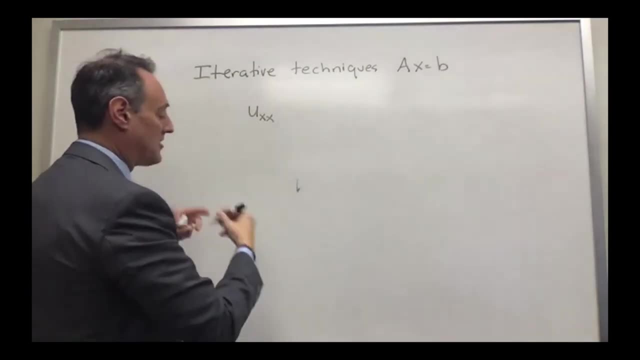 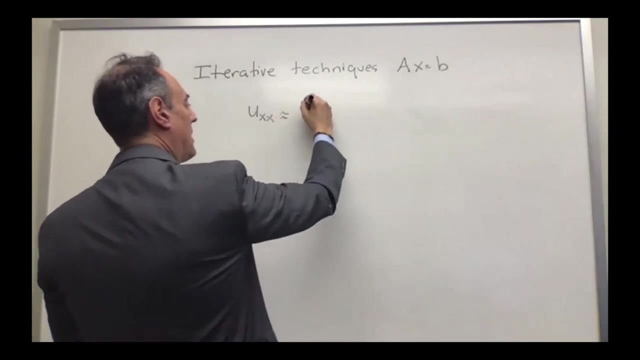 If you were to take a vector u and you take two derivatives of it, then if I discretize this, the two derivatives, the second derivative formula, and I'm not going to go into details here, but it looks like something like this: 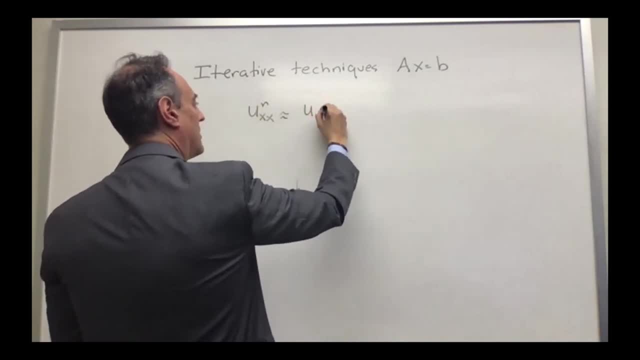 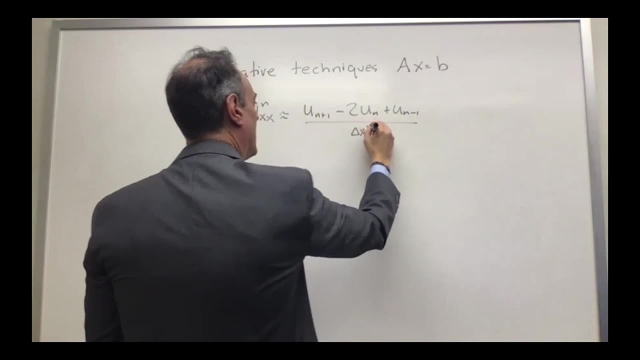 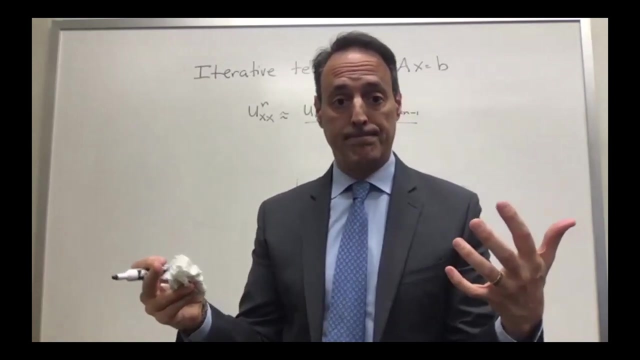 If I'm at the nth point, it's basically point front minus twice this point plus point behind over delta x squared. This is an approximation to the second derivative, Using just your slope formulas, essentially, But what does this look like in terms of a matrix? 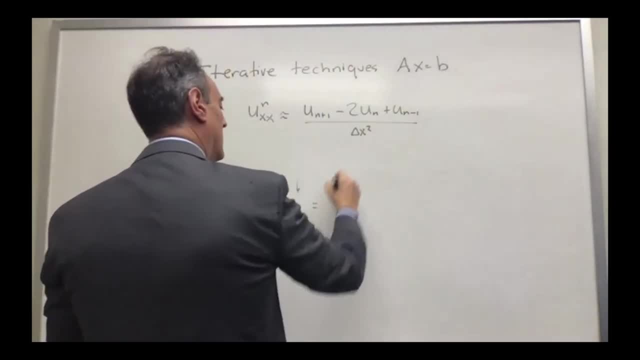 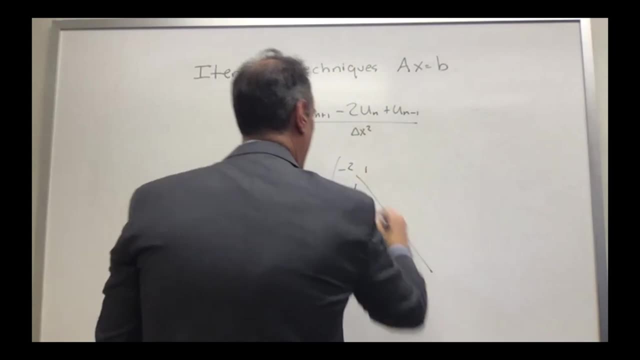 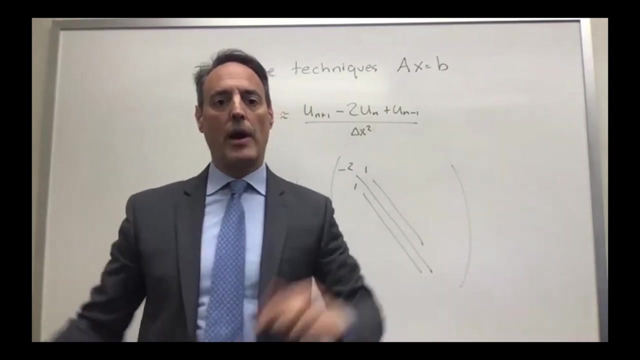 Well, in terms of a matrix, a second derivative matrix looks something like this: It's 1 over delta x squared negative, 2 down the diagonals and 1 on the off-diagonals, Zero everywhere else. And these kind of matrices show up everywhere. 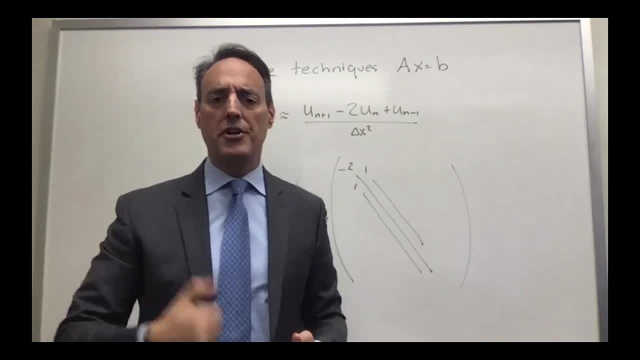 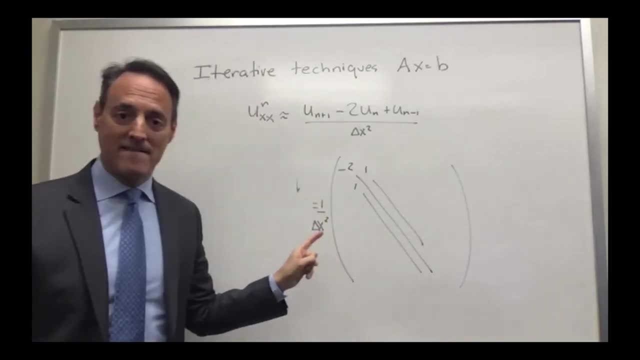 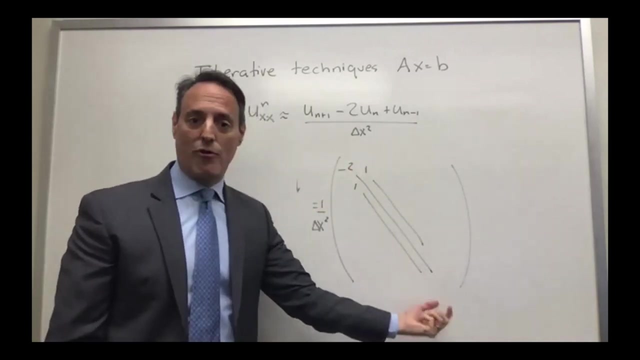 because they're coming from physics and coming from engineering problems, where you say I'm going to do this, where you say I'm going to solve this problem. so I have this massive matrix, but notice the structure. in fact it's almost all zeros and it's got this tri-diagonal form. and remember what we tried to. 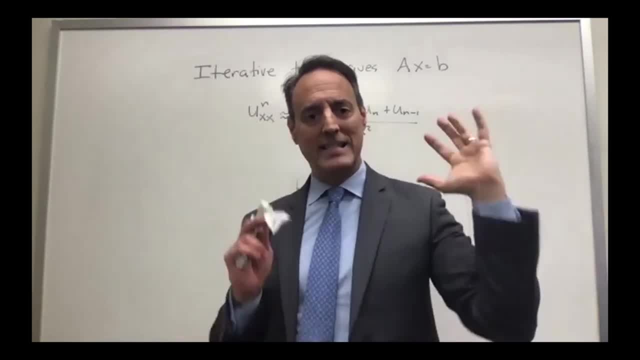 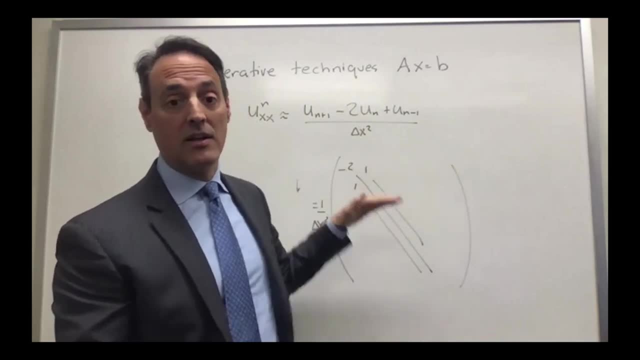 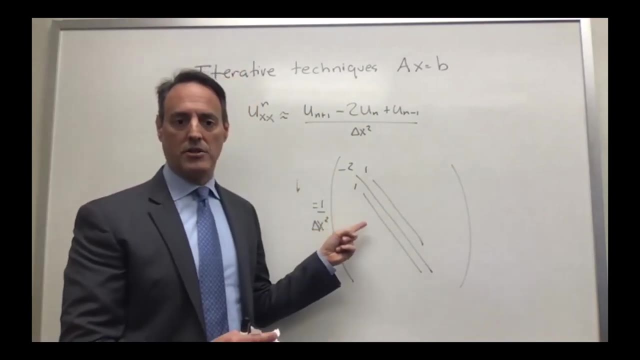 do when we solved these for the eigenvalue problem. step one: try to reduce your matrix to like tri-diagonal form or, in the case of the SVD, bi-diagonal form. step two: iterate to the solution. I've already got this thing as a differentiation matrix in tri-diagonal form, and then you ask: okay.